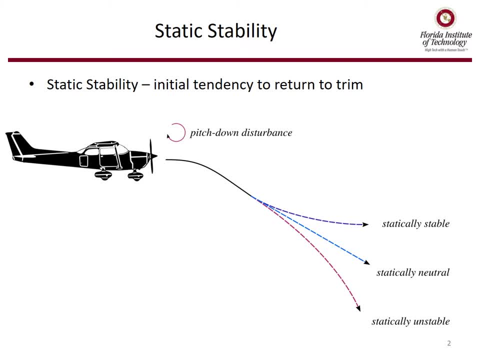 illustration. here the airplane is flying straight and level and then it gets a pitch-down disturbance. So we want to look at what's the initial tendency after the disturbance. We can see that the purple behavior shows the airplane trying to get back to level flight. so its initial tendency is to get back to 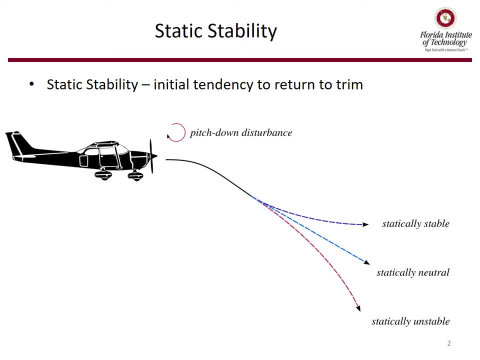 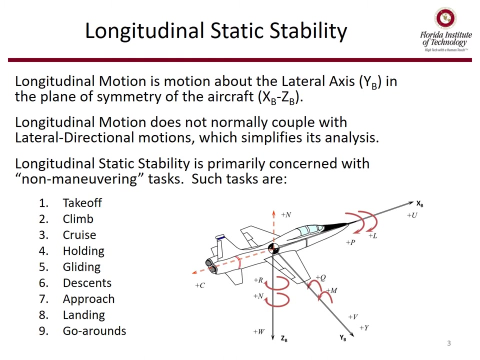 trim. The light blue line shows that the airplane, after the disturbance, just wants to continue down that straight track, so that's statically neutral. And then we see the pink line that, after the disturbance, the nose of the airplane wants to continue to go down further, which means it's statically unstable. So 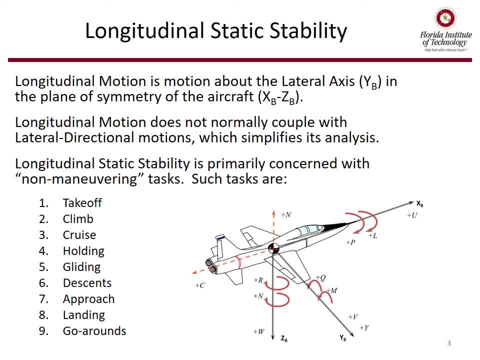 now we'll distinguish between just static stability and longitudinal static stability. When you're flying in an airplane, the longitudinal motion is pretty much when you push forward on the stick, pull aft on the stick. It's motion about the lateral axis, the YB axis, and the motion is in the plane of symmetry. 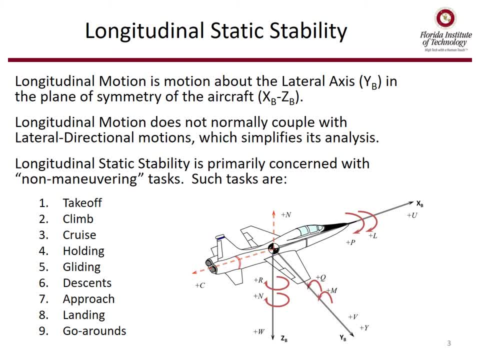 of the aircraft, the X-body, Z-body, plane of symmetry. So this is a confusing point. It's longitudinal motion, but it's motion about the plane of symmetry of the aircraft: the X-body, Z-body plane of symmetry. So this is a confusing point. It's longitudinal motion, but it's. 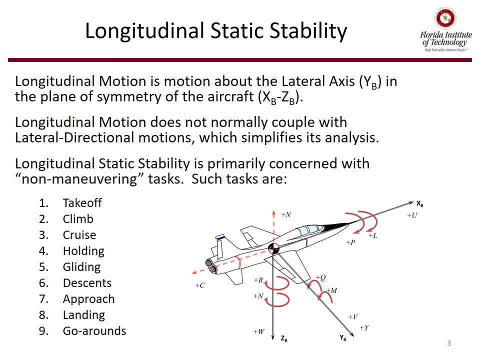 motion about the lateral axis, the Y-body axis, out the right wing. Now, the good thing about longitudinal motion is it doesn't couple with the lateral directional motion, which simplifies its analysis. The types of maneuvers that we want to look at- longitudinal static stability- are really maneuvers that. 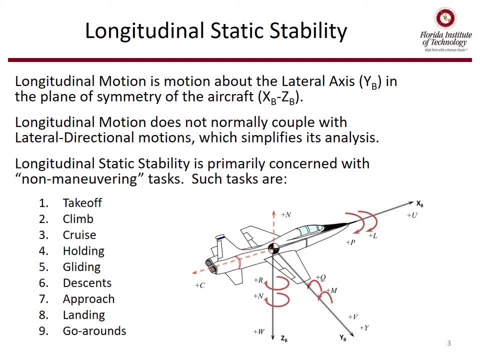 don't really maneuver at all, or non-maneuvering tasks, Things like takeoff, climb, cruise. These are fairly simple maneuvers, Fairly steady things that we do. we are confessing the aircraft. we're not yawing the aircraft, just raising the nose a little bit pushing. 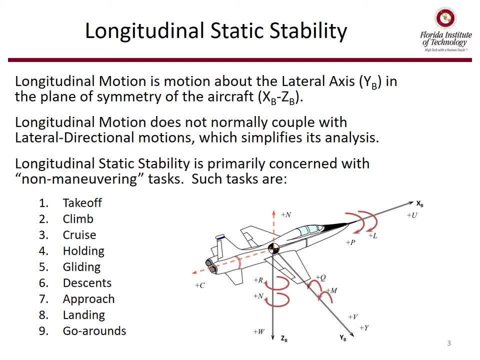 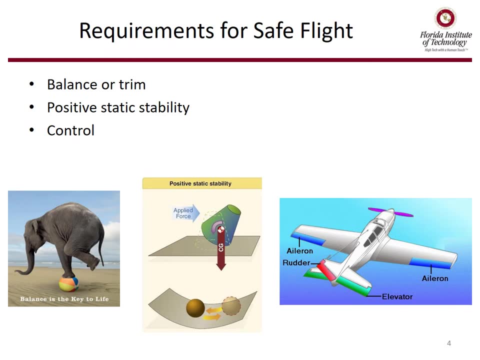 the nose down a little bit. Takeoff, climb, cruise, gliding, descent approach- These are all longitudinal static stability maneuvers. To fly an aircraft safely, we need to be able to balance or trim the aircraft. your needs to have positive static stability and then we have to be able to control. 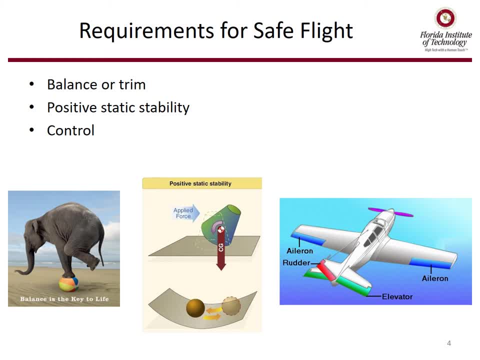 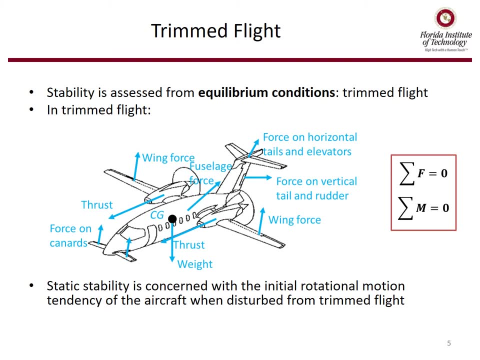 the aircraft Stability is assessed from an equilibrium condition, in other words a trimmed flight condition, And mathematically the airplane is trimmed or balanced when the sum of the external forces is zero and the sum of the external moments are zero. And so we look at the airplane in the diagram and we 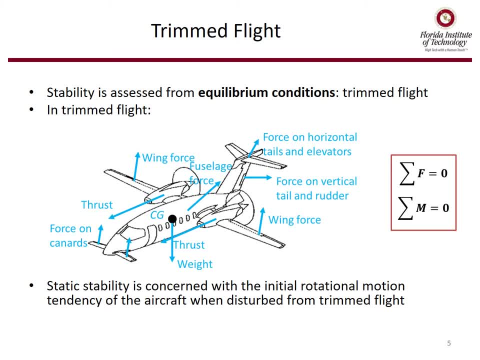 see all these forces, and some of the forces go forward, some go back, some go up, some go down, But the sum of the forces have to cancel out and basically go to zero, and then the moments generated have to also sum to zero. 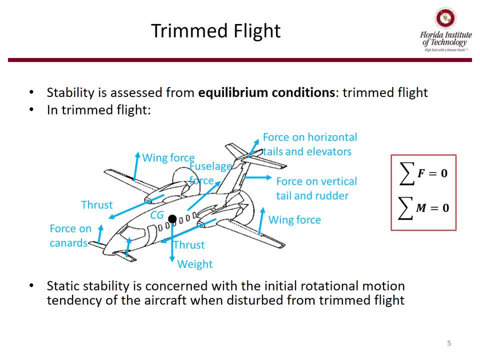 Static stability. again we're concerned with the initial rotational motion tendency of the aircraft. Static stability is the force that is applied to the aircraft after it's disturbed from a trimmed flight condition. Pilots think a trim means I can take my hands off the controls. the airplane is balanced. 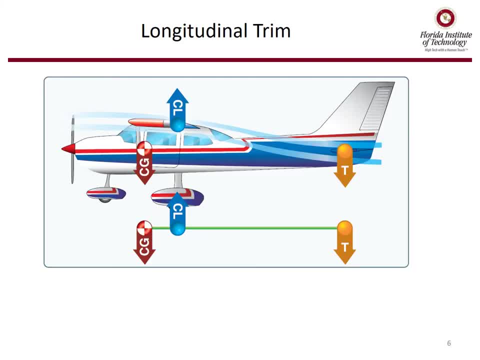 Now let's look at longitudinal trim. So here's an aircraft flying straight and level. It has a center of gravity called CG and that's where the weight vector acts. main wing generates lift. You can see this: CL, that's the coefficient of lift generated by the main wing, And then you see a downward 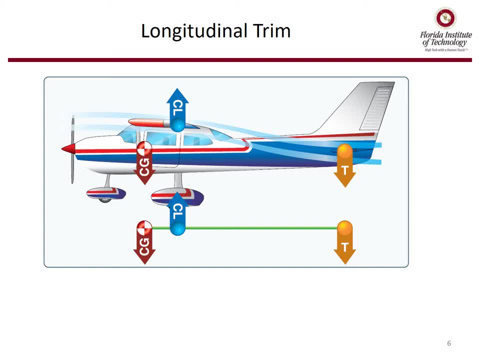 vector of the tail lift. So when we sum the moments about the CG, we look at the forces by the main wing and the force by the tail and they have to balance. So the main wing generates upward lift and it's at a short distance from the CG. 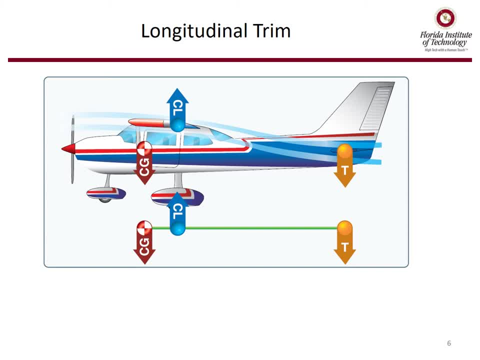 And the tail needs to counter that with a downward lift and it's at a longer distance from the CG. So the tail doesn't need as much lift because it's at a longer distance, but it still needs to counter or balance the lift from the main wing. 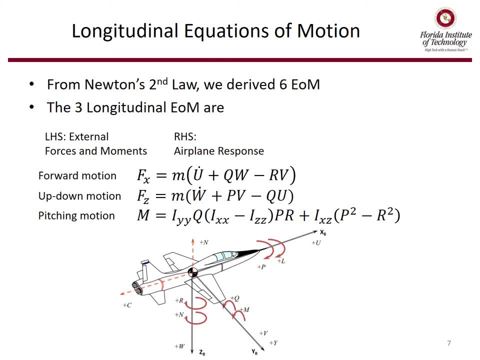 In the introductory lesson in chapter 19,. we talked about the equations of motion. We derived those from Newton's law and we derived six equations of motion. We rearranged them and we came up with three longitudinal equations of motion and they're listed here. Let's just go over. 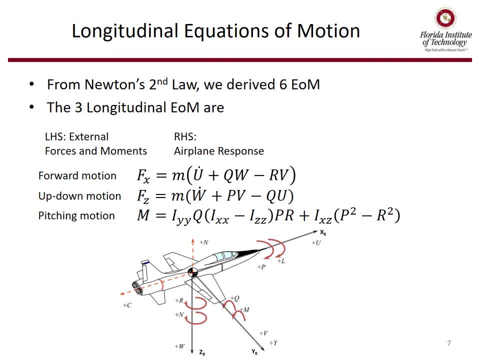 again what these are made up of. The left-hand side are the external forces and moments that are generated on the aircraft. The right-hand side is how the airplane responds And we have all the different things. we define Forward speed, side speed, downward speed. We have pitch rate, roll rate. 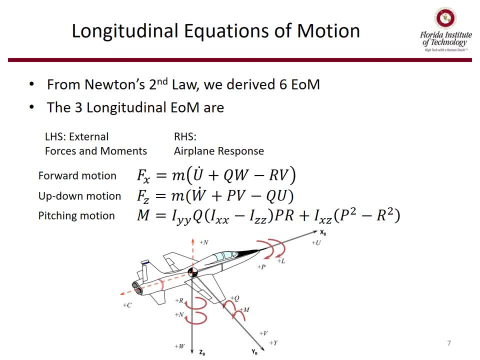 yaw rate. We have moments of inertia, products of inertia mass. All of these parameters were defined in our opening lecture And that's all the airplane response on the right-hand side of the equation. Let's now focus on the left-hand side. We have forward. 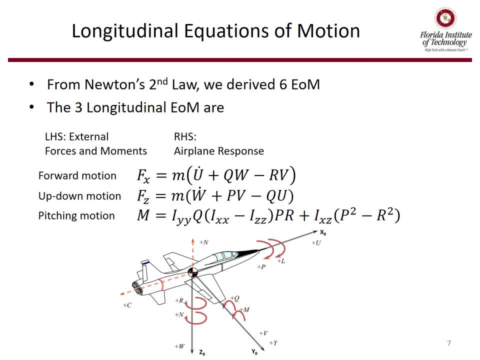 motion, and so there's going to be forces in the x direction, up down motion, forces in the z direction, and then rotational or pitching motion, which was denoted by the symbol m, And that's rotation about the y-body axis, That's up-down rotation, nose-up, nose-down rotation. When we 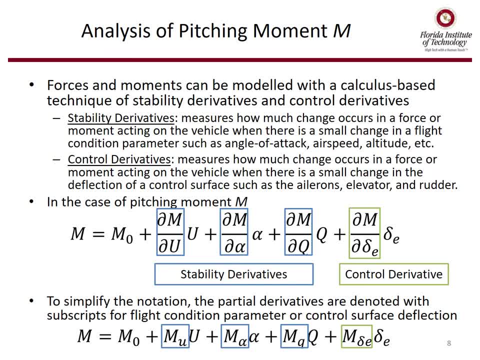 analyze pitching motion or the pitching moment m. we're going to use a calculus based technique that has stability derivatives and control derivatives. So the stability derivatives: they measure how much change occurs in a force or moment acting on the airplane. when there's a small change in a flight, 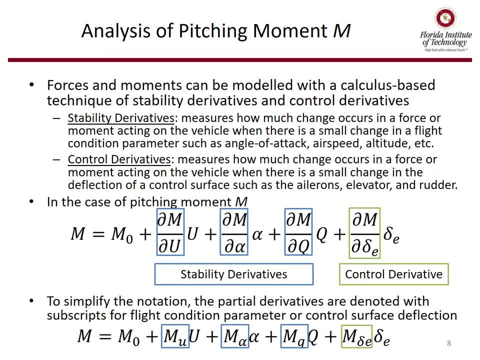 condition parameter, such as angle of attack, airspeed, altitude, etc. Control derivatives, on the other hand, they measure how much change occurs in a force or moment acting on the vehicle when there's a small change in the deflection of an actual control surface, such as the aileron, the elevator or the rudder. In 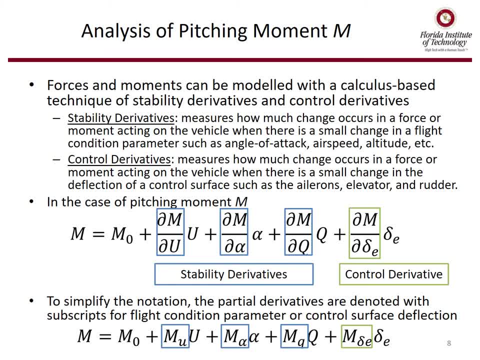 the case of pitch motion or pitch moments, we measure how much change occurs in a vehicle. So the stability derivatives measure the mental state of a vehicle when the vehicle is paving its way off the ramp and when it takes off the ramp. So the z-levels are what generate the moment delta e. So the calculus based 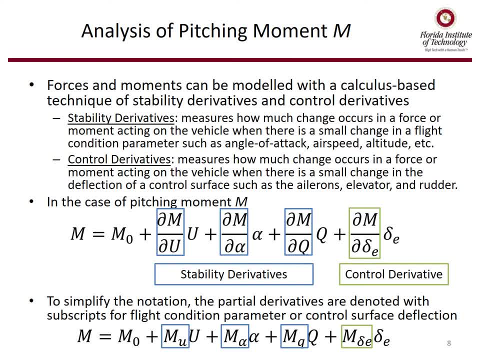 model uses the stability and control derivatives and it breaks down the moment on the left-hand side of the equation into these sub-elements. So there's a moment with zero angle of attack angle of attack, then there's the moment due to pitch rate, etc. So this is the calculus-based. 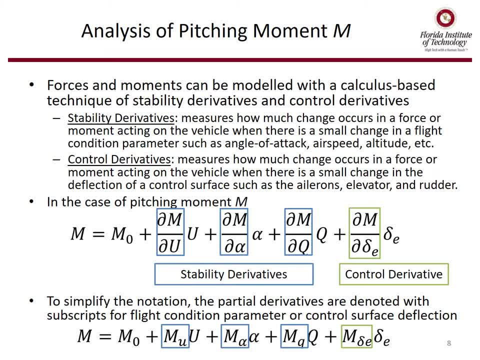 model of using stability derivatives and control derivatives. All of this builds to that one m on the left-hand side of the equation on the previous slide. Now all these partial derivatives- partial m, partial u, partial m, partial alpha, etc. makes the notation somewhat cumbersome. 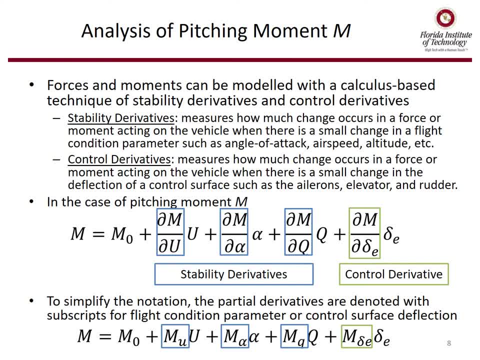 So to simplify the notation, they replace the partial derivatives with this subscript notation. So instead of saying partial m, partial u, it's just m sub u. Likewise, partial m, partial alpha is m sub alpha. So this is a way to analyze pitching moment or aircraft motion using a. 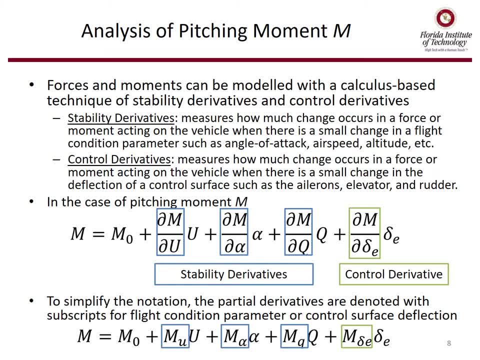 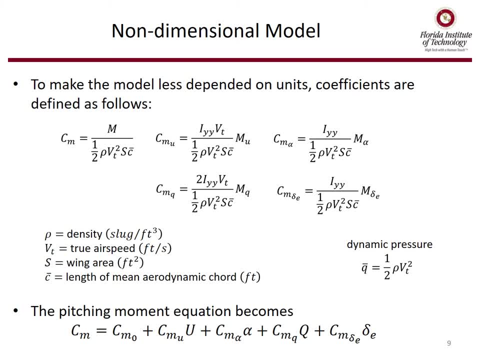 calculus-based technique called stability derivatives and control derivatives. To make the model on the previous slide less dependent on units, they've developed coefficients that are non-dimensionalized, And so instead of moment, we're going to have the coefficient of moment c sub m, And you can see it's the pitching moment m, and then we divide it by 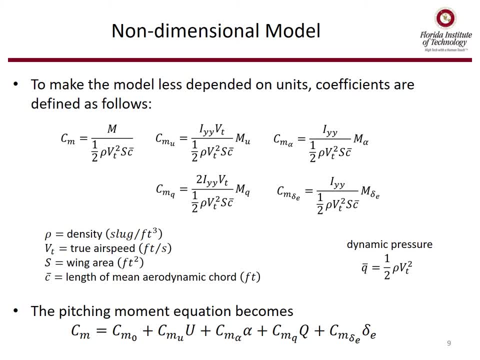 some parameters that make it non-dimensional, And in this case it's one half rho, which is density, v, true, which is true airspeed, squared capital S, which is the wing area, and a term called c bar, which is the length of the mean aerodynamic cord. 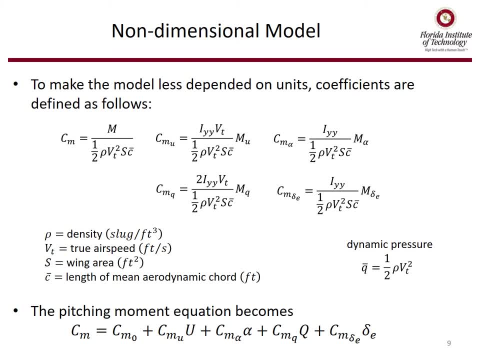 So the stability derivative m sub u then now in coefficient form becomes c sub m sub u and it still has mu, and then it's non-dimensionalized by the same denominator. and it also has a moment of momentum which is c sub m, and then it's non-dimensionalized by the same denominator. 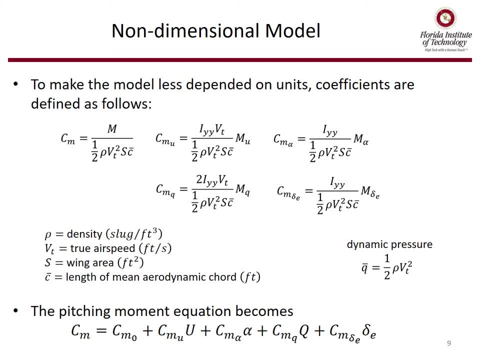 and a true airspeed in the numerator. So this is an established practice that aerodynamicists have done to basically take the model on the previous slide and make it non-dimensional using these coefficients as we've defined here. So one other thing you'll see sometimes is, instead of writing one half, 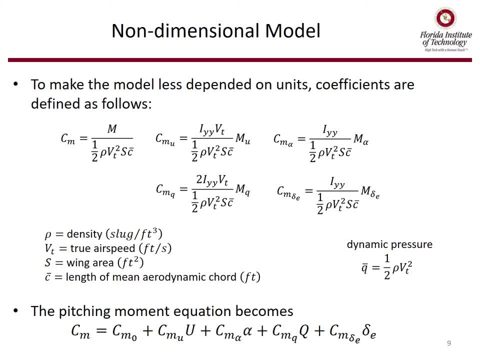 rho v true squared. they'll just use dynamic pressure. q bar is the same thing as one half rho v true squared. So sometimes you'll see the coefficients listed with q bar instead of one half rho v squared. But when you do this 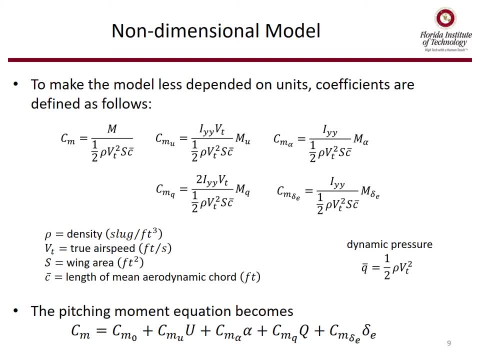 the equation in the previous slide then has a coefficient form at the bottom of the page. So the moment coefficient is c m zero plus c m u times u plus c m alpha, times alpha, etc. It's the same type of equation. it's just now. we have non-dimensional coefficients. 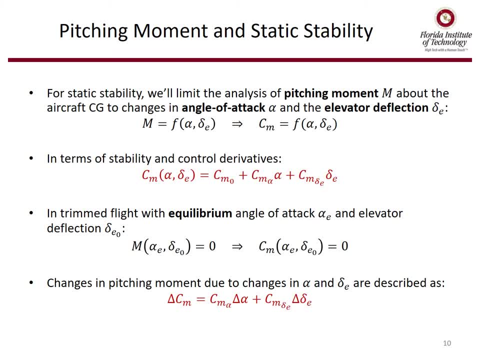 We already said that the pitching moment m really has a function of a lot of things: forward speed, angle of attack, pitch rate etc. But for static stability we're going to limit the analysis of pitching moment to really the impacts of angle of attack and elevator alone. We're going to ignore. 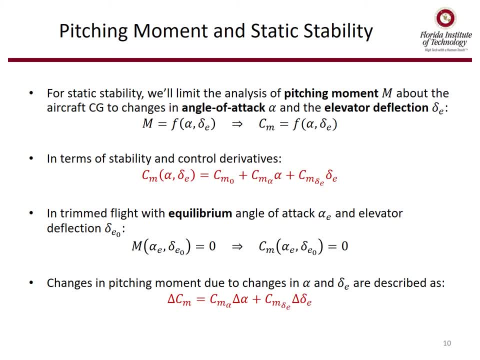 forward speed and pitch rate etc. And for static stability it's just the pitching moment due to angle of attack and elevator deflection. So we can take the equation on the previous slide and just simplify it, drop the terms that don't matter, the c m u, u and the c m q q- and we're down to now. 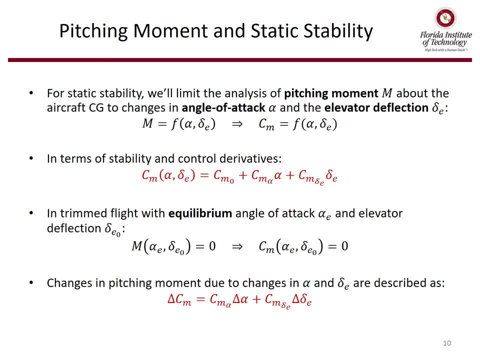 three terms. on the right-hand side Now, when we trim the aircraft hands off, it's going to be a certain angle of attack and a certain elevator. that got us to the trim condition. But in trim flight the pitching moment is zero and the coefficient for pitching moment c m is zero. So 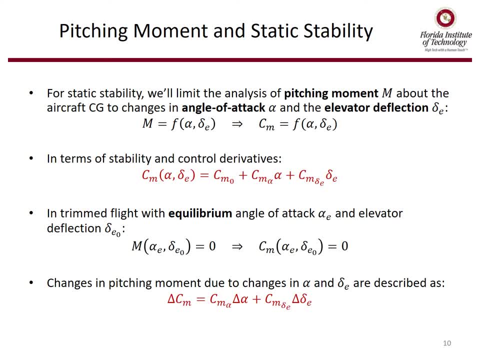 if we trim the aircraft hands off, it's going to be zero. Now we're trimmed and we want to analyze the motion of the aircraft due to a disturbance or a change in some variable. So the bottom equation is a change in pitching moment due to a change in angle of attack or a change in 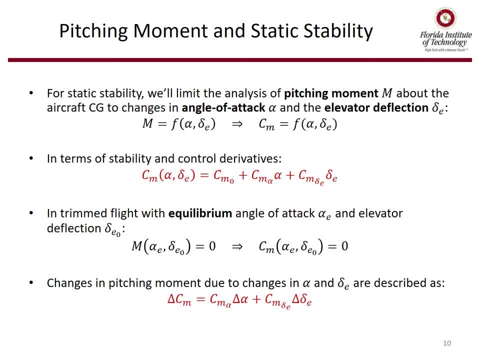 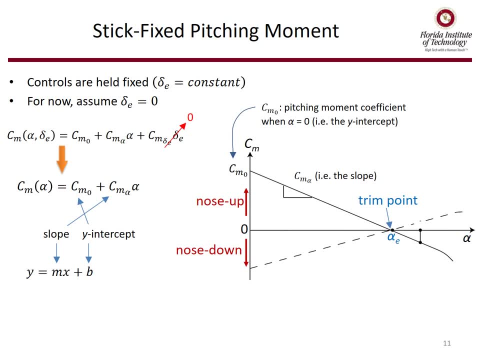 elevator deflection. When we look at the pitching moment, there's two cases: Stick free and stick fixed. We're going to start with a stick fixed case, So the control positions are held in a fixed position. They're constant. The elevator deflection is constant in this case. 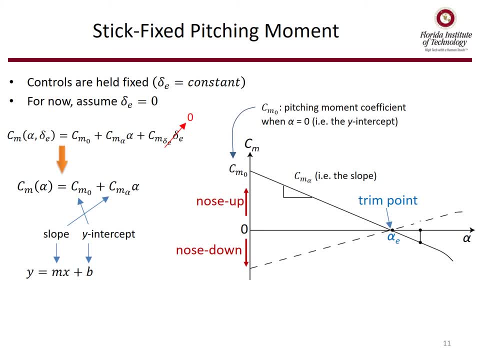 For lack of a better value. let's just assume it's zero. Zero is a constant number. It won't change the analysis, but right now it'll make understanding the concept a little simpler. if we make the elevator zero, It drops that third term. 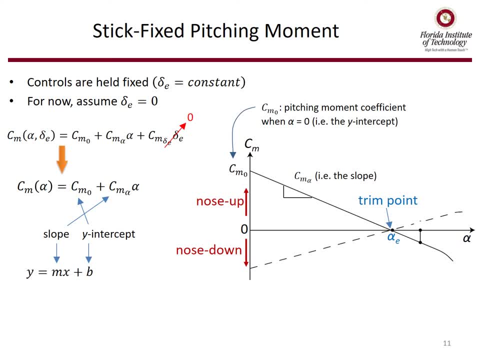 What we get then is the classical high school algebra: y equals mx plus b type of relationship, a linear plot. So there's going to be a slope and there's going to be a y-intercept, In this case the y-intercept. 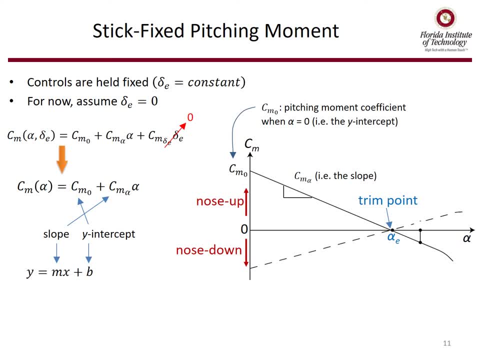 is c m sub zero. It's the pitching moment coefficient when the angle of attack is zero, but it's really the y-intercept. And then we have c? m alpha times alpha. The c? m alpha portion is the slope of the line, the change of y over the change of x. 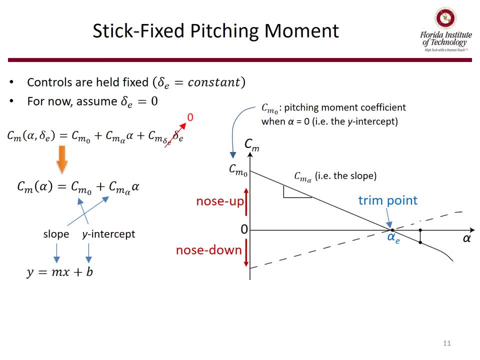 On the graph shown on the right, you can see that that slope is negative. So we have a positive y-intercept, a negative slope, and then the line eventually intersects the x-axis. When it intersects the x-axis, the overall pitching moment, the y-axis value now, is zero, which means the airplane is. 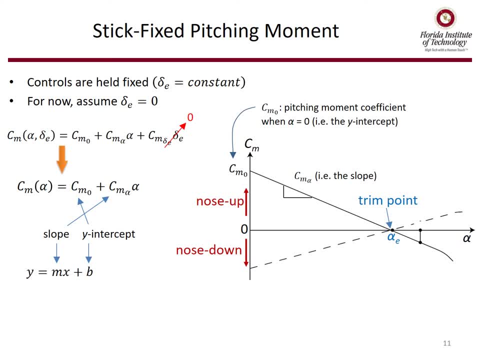 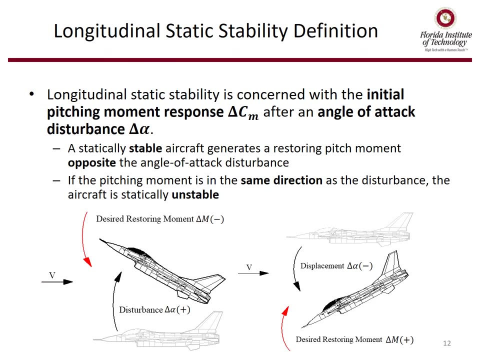 trim. There is no pitching moment, And so that angle of attack, which is the x-axis that got us to that point, is the trim point or it's the trim angle of attack. alpha, sub e. Longitudinal static stability is concerned with the initial pitching moment response, that delta. 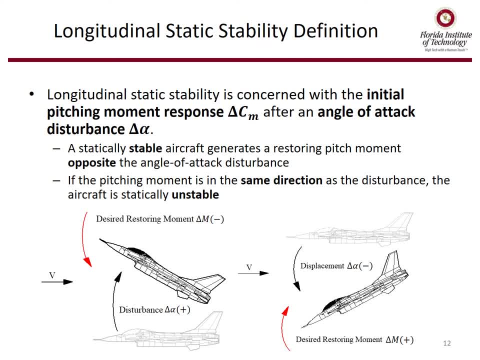 pitching moment. when there's a disturbance in angle of attack, or delta alpha, A statically stable aircraft will generate a restoring pitch moment opposite the angle of attack disturbance. What do I mean by this? So if I have an angle of attack of, say, 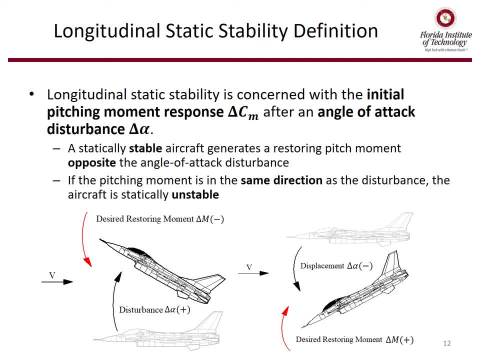 six degrees and then I get bumped to eight degrees. well, we want the airplane to push the nose back down to go back to the trim angle of attack of six. Likewise, if I'm trimmed at six degrees angle of attack and a gust pushes me to two degrees, 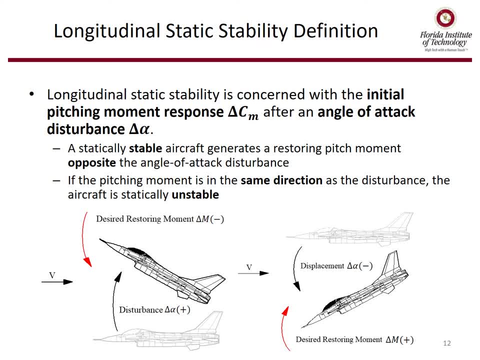 angle of attack. I want the nose to come up, then the natural restoring moment to come up, to get back to six degrees angle of attack. That was my trim value of angle of attack. So again, we want the restoring moment to be in the opposite direction of the disturbance. 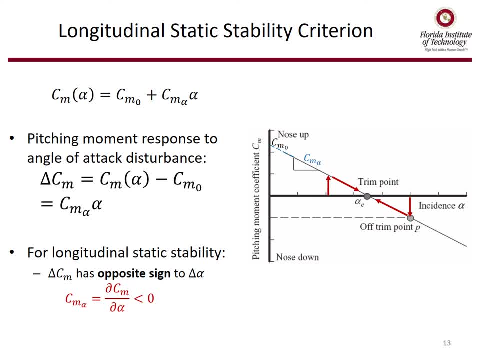 Another way to look at that is going back to the CM versus alpha curve, the linear relationship we showed earlier. Again, we said when that curve crosses the x axis, that's the trim point, that's the angle of attack that was needed to be in the rest of the plane. 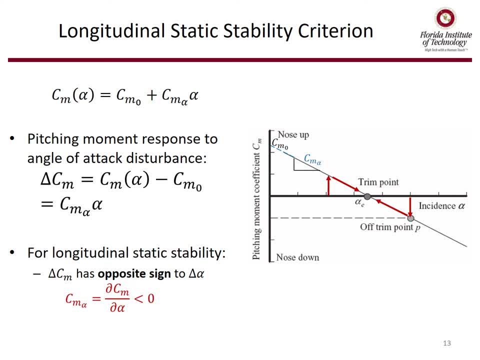 to trim the aircraft to have zero pitching moment. In this example, alpha E. if we get a disturbance in angle of attack, that makes the overall angle of attack larger. so let's say again: alpha E was six degrees. If we go larger that means we're to the right of alpha E. 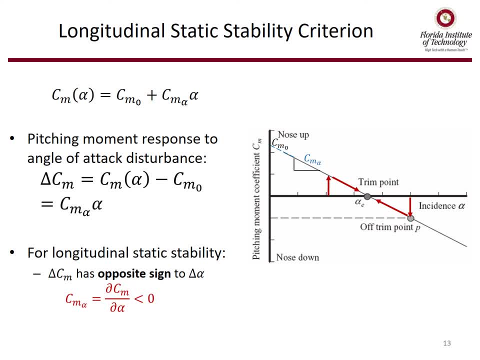 at something like eight or 10.. And if we look at the plot, it means that we need a negative pitching moment. We've got to think of the right-hand rule in this case. right, The YB axis is going out the right wing. 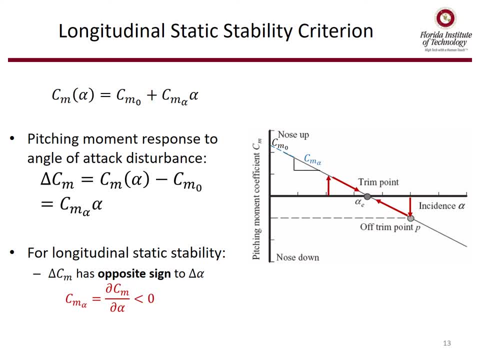 And so a negative pitching moment using the right-hand rule would push the nose down and get us back to six degrees angle of attack. Likewise, if I'm at six degrees angle of attack and I get pushed to a lower angle of attack like four, 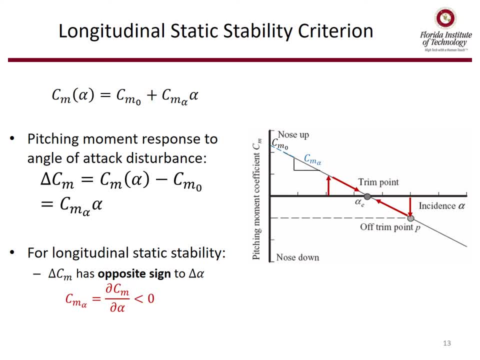 that's equivalent of going left on the axis from our alpha E. That puts me at a positive pitching moment, which is going to push the nose back up and get back to six degrees angle of attack. So whether we look at it from pictures on nose up, nose down, 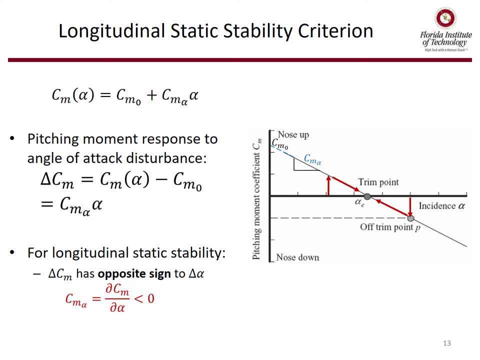 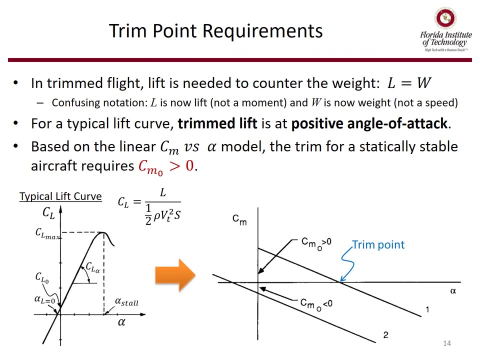 or we look at it on the plot. it's still basically telling us that for positive static stability that slope CM alpha has to be negative. When we trim an aircraft in level flight, the overall lift of the aircraft has to balance the overall weight of the aircraft. 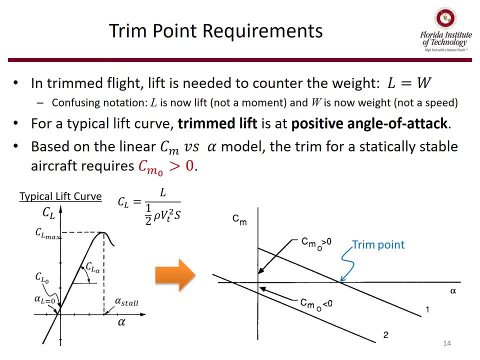 Otherwise we would climb and we would have a negative 10%. So lift equals weight if we trim in level flight. Now this starts to cause confusion in the notation. Earlier we defined L as a moment and we defined W as a speed. 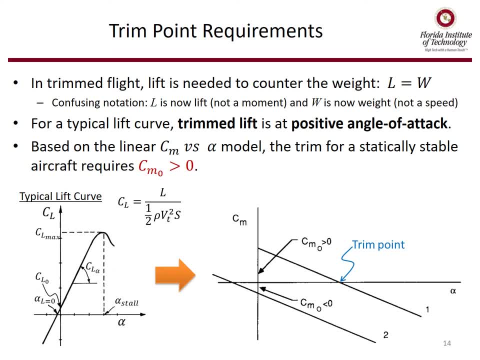 In this case, L is now lift, not a moment, and W is now weight, not a speed. This is confusing, But unfortunately we're stuck with these variables in this nomenclature and they do use certain rules, and we're forced to rely on the context of the problem. 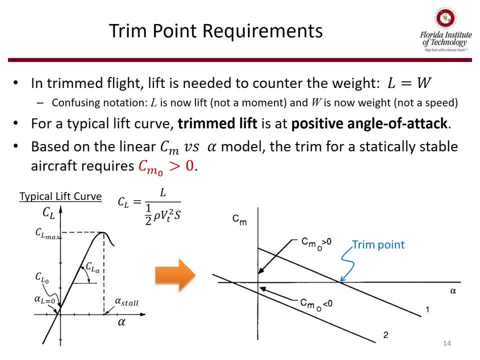 or the equation to understand which letter means what. Let's now look at a typical lift curve. This is one of the basic curves that any aerodynamic book starts with. It's a coefficient of lift. CL is the y-axis and alpha, or angle of attack, is the x-axis. 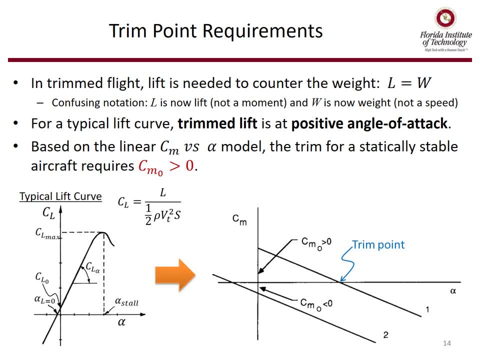 and a typical lift serve is shown on the lower left portion of the slide. Again, CL is defined as L, in this case lift divided by one: half the density times the true airspeed, squared times the wing area. That's a classic definition of what CL is. 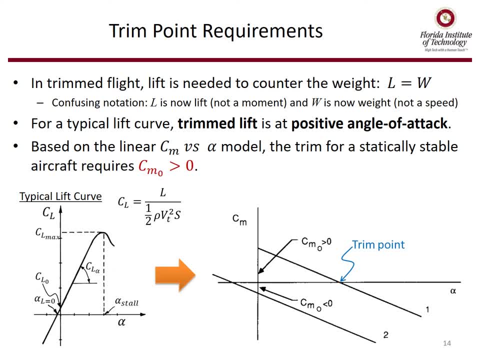 the coefficient of lift. We see, then, for an aircraft to be trimmed in level flight, it needs to have a positive angle of attack. So, based on this linear relationship of CM versus alpha model, the trim then for a statically stable aircraft is also going to require that that y-intercept, that CM0, also be 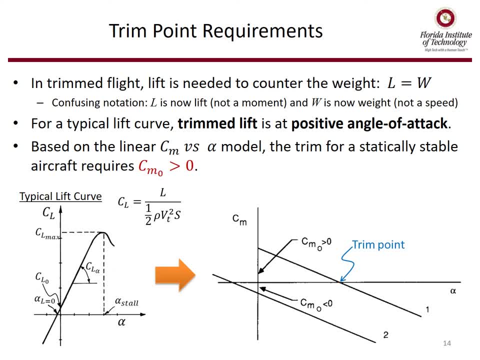 positive. On the plot on the lower right of the screen you see two CM versus alpha lines. The top one has a positive CM0, or positive y-intercept and we're able to cross the x-axis at a positive angle of attack. The lower curve: 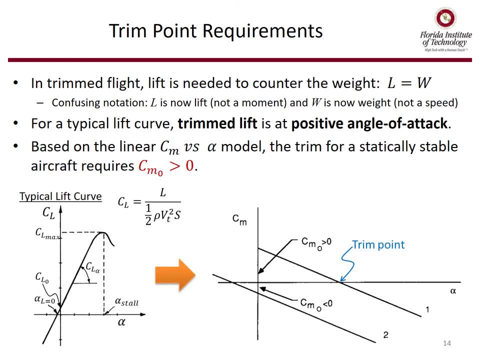 has the same exact slope but its y-intercept is negative and we cross the x-axis at a negative angle of attack. That's not possible based on the CL versus alpha relationship and the CM versus alpha model. Again, we want a positive CM0, or positive y-intercept and we need a negative slope. 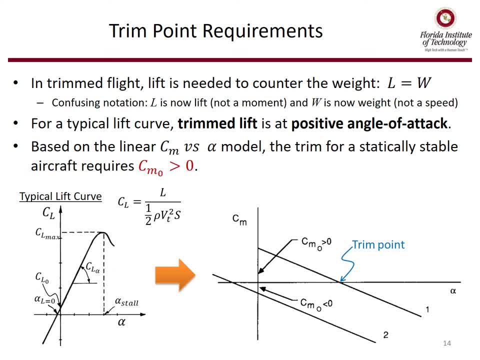 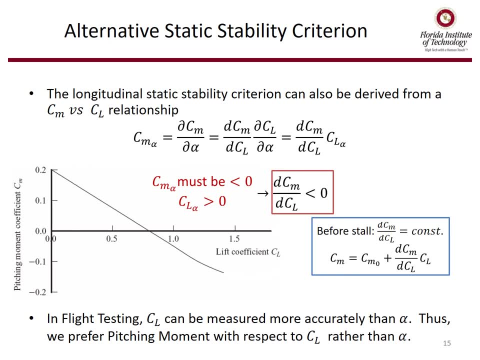 for static stability In flight. test angle of attack is negative and we need a negative slope for static stability In flight. test angle of attack is negative and we need a negative slope for static stability. We look at that slope as辜0.. 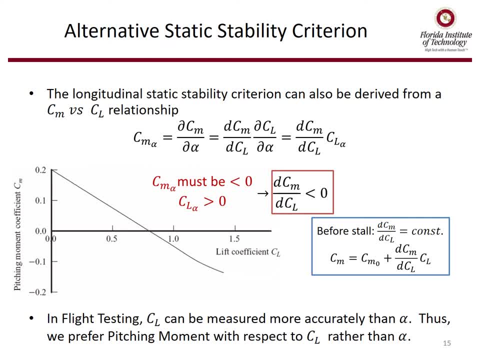 We may want to look at our analysis based on something. CL is actually something we measure quite easily in flight. I can take the relationship for static stability- that the fact that CMa needs to be negative– I can derive an equation or another relationship that gives me another slope that I can measure. 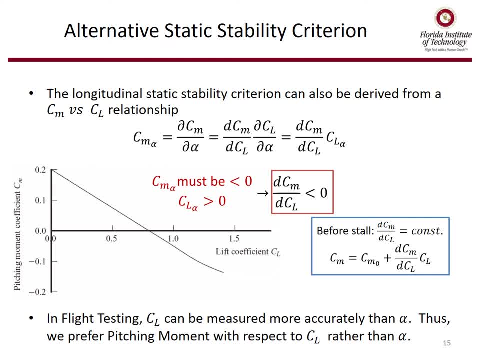 in flight We can forget the balance, but its labels doSmoles. that is the same again. Here's the analysis. We have a definition for CM alpha. It needs to bone down in a natural way. I want to make sure thisалист is in line with the disadvantage of Oct premises. 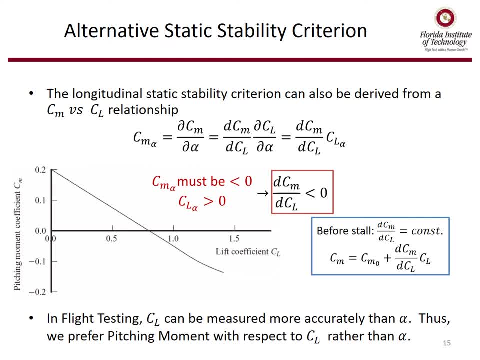 and basically we multiply the numerator and denominator by partial CL and we get a new mathematical definition now that CM alpha is nothing more than DCM divided by DCL times, CL alpha or the lift, the CL versus alpha slope. And we know that's positive from the previous slide. 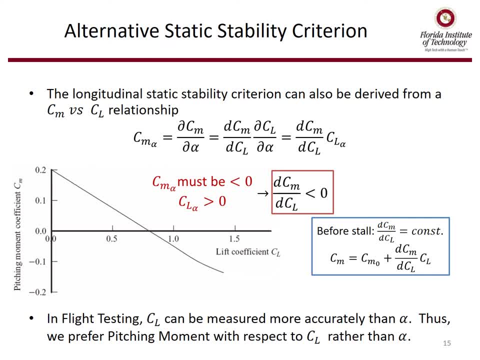 The bottom line is we need CM alpha to be negative And in this problem that also implies that DCM over DCL must also be negative. And again, we do this because we can measure CL easily in flight. It's more accurate than angle of attack. 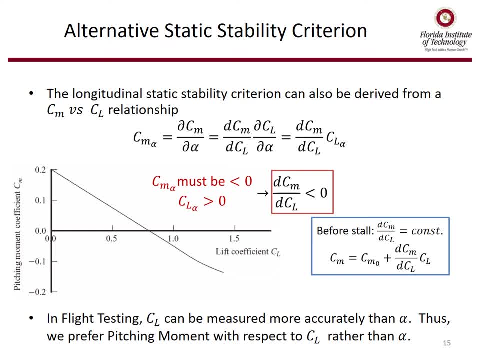 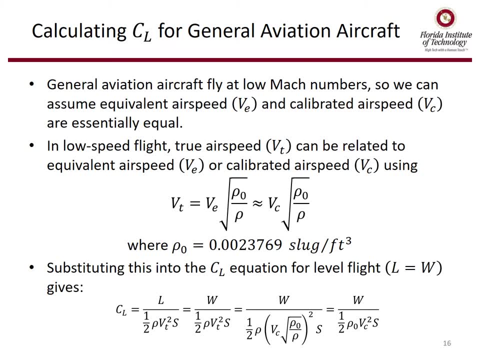 And sometimes we just don't have angle of attack. So how do we measure CL in flight? Well, for general aviation aircraft, we fly at low Mach numbers, And so we can assume that our equivalent airspeed and our calibrated airspeed are essentially equal. 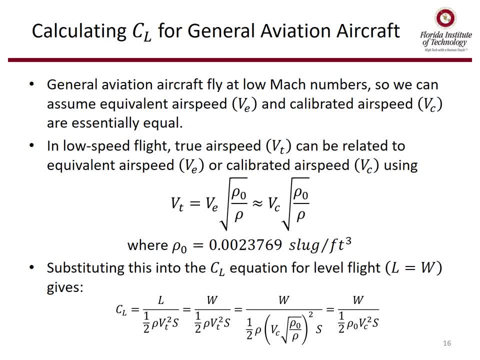 That being said, I also have an equation now that relates equivalent airspeed to true airspeed, and that's the equation shown there. a true airspeed is the equivalent airspeed divided by the square root of the density ratios. Rho. sub zero being the C-level, density got a constant value. 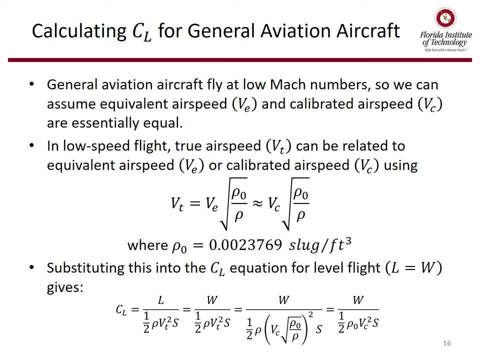 0-point 0023769 slugs per foot cube Density is whatever the density is at altitude. So since the equivalent airspeed and calibrated airspeed are, October can also be going before. I could say that in 1927, with theither slide hitting 항상 positive. So we be reach million filling ThisAtcom And I also have the, the Equivalent AirSpeed ratio, Rho sub zero being the C level density And that's a constant value. Zero point. 0.0023769 slugs per ft cubed Density is whatever the density is at altitude. 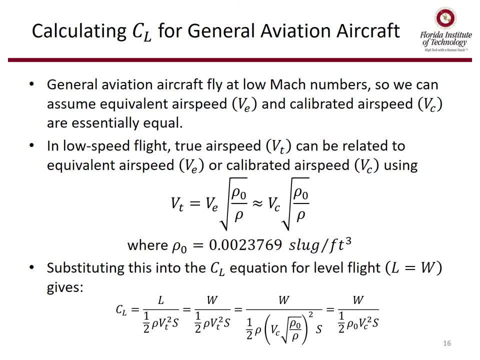 calibrated airspeed are about the same. at low flying general aviation aircraft we can replace true airspeed with calibrated airspeed times, the square root of the density ratio. Now, if I substitute that in our lift equation- and since I'm in level flight I know that lift. 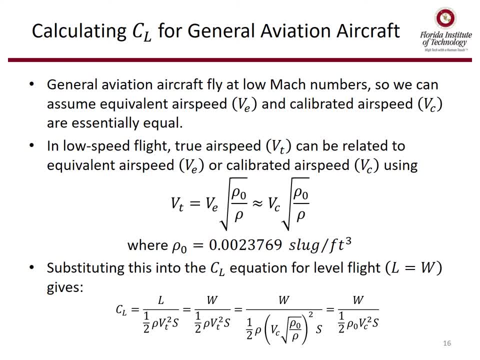 equals weight And I can always- I always- know my aircraft weight based on the fuel burn and our empty weight and our weight and balance at the beginning of the flight. I know the weight. then all the way to the right-hand side of the equation, I know weight. 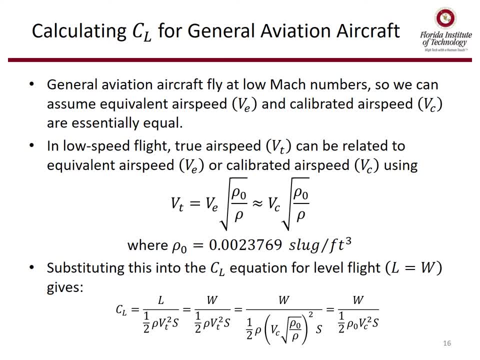 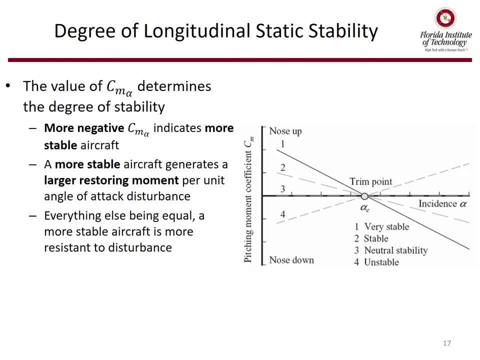 sea level. density is a constant value. I know my calibrated airspeed and wing area doesn't change, So I'm easily able to calculate CL based on my weight and my calibrated airspeed. The other numbers are constants. So we said that CM alpha, or that slope, has to be negative for stability. 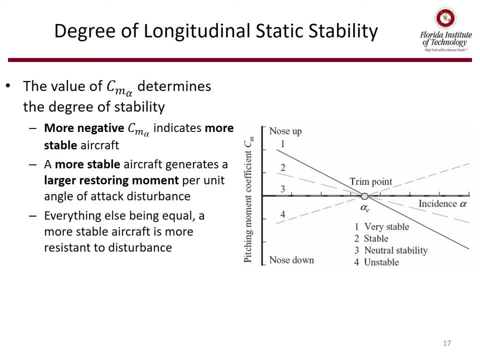 And we can look at it now in terms of the degree of stability. So obviously the more negative the slope, the more stable the aircraft. So number one on the plot shows you the most stable aircraft. A more stable aircraft generates a larger restoring moment when its angle of attack is disturbed. 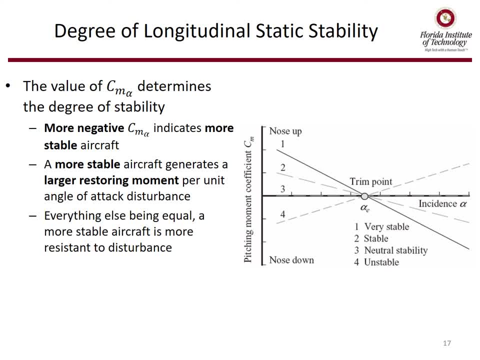 So, everything else being equal, a more stable aircraft is more resistant to disturbances. Now we have some other slope shortcomings Shown on that plot. to the right we have slightly less negative slope in the number two curve. We have a zero slope in the number three curve. 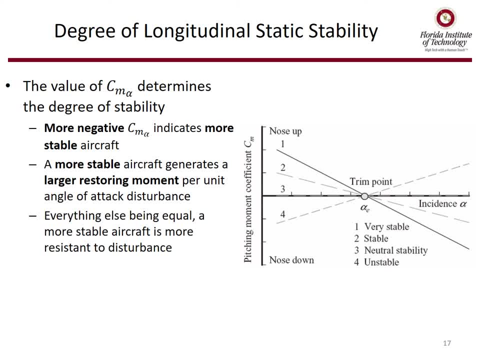 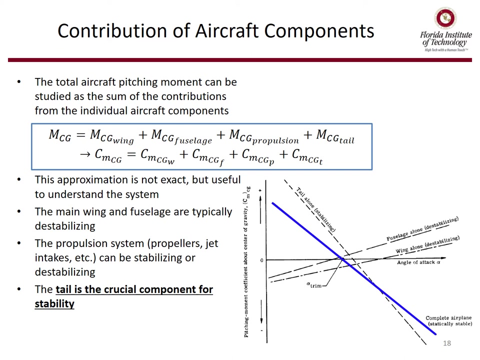 and then we have a positive slope in the number four curve. So in the number four curve is statically unstable. The number three curve is neutrally stable and two and one are stable curves where one's being more stable than the second. So when we're looking at total aircraft pitching moment or the left-hand side of the equation, 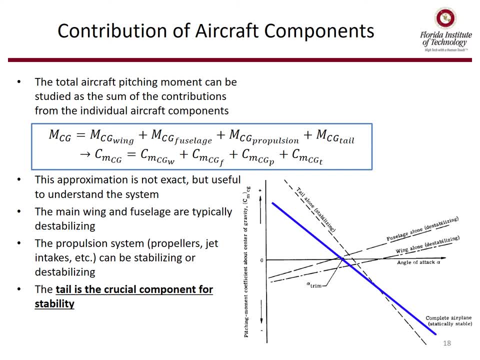 we can kind of look at the sum of the individual aircraft components. In other words, the aircraft has a wing component, a fuselage component, propulsion components and the tail component. So we can break them down one by one And yes, this isn't exact. 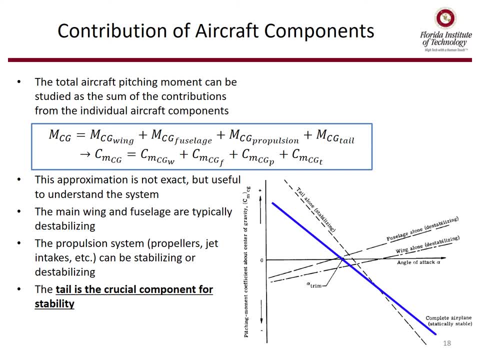 It's a model, but it's actually useful for the understanding of the system. So we see in the graph on the lower right is you can see the different subsystems broken out. The wing alone has a positive slope that's destabilizing. The fuselage alone has a positive slope that's destabilizing. 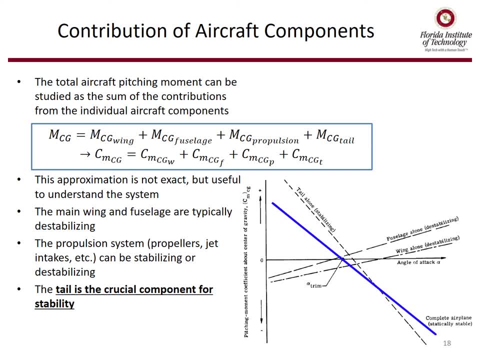 And so the main contributor to overall aircraft stability looks to be that tail. The tail alone is what gives us that strong negative slope that overcomes the other positive slopes. So other systems like propulsion systems, where the propellers and the jet intakes, et cetera. 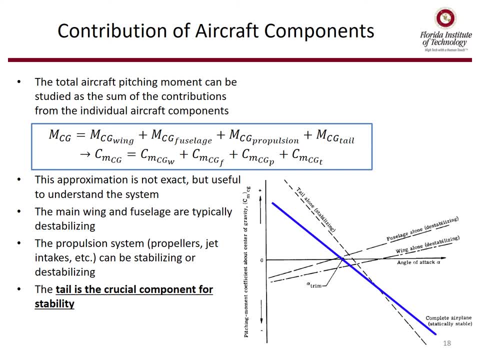 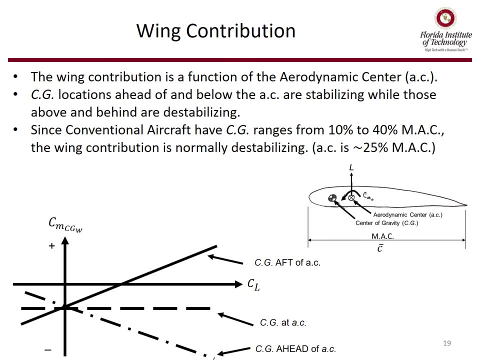 sometimes they're stabilizing, sometimes they're destabilizing And even sometimes the main wing can be stabilizing or destabilizing. We'll talk about those here in the next couple of slides. The main wing: The main wing generates lift at the aerodynamic center. 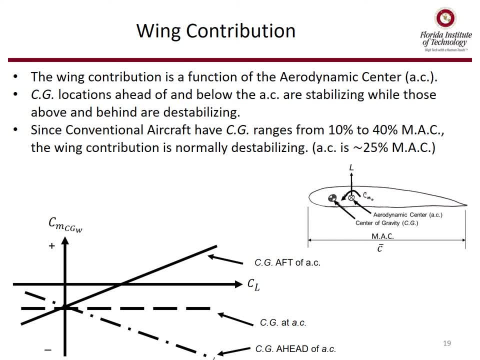 At zero angle of attack. it can also generate that initial pitching moment. CM And the aircraft will have a center of gravity based on where the baggage and the passengers and the other equipment are. The center of gravity moves. It can move as much as 10% of the mean aerodynamic cord to 40% of the mean aerodynamic cord. 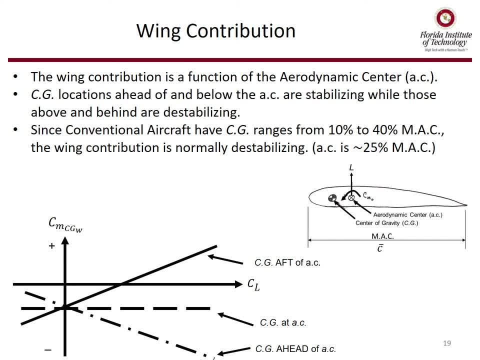 The lift of the main wing, however, typically acts at 25% of the mean aerodynamic cord, as shown in the diagram. But again, CG can move based on fuel burn, based on baggage, based on passengers, And so sometimes the main wing contribution has a stabilizing effect. 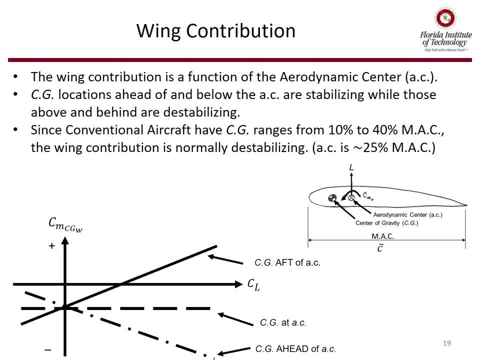 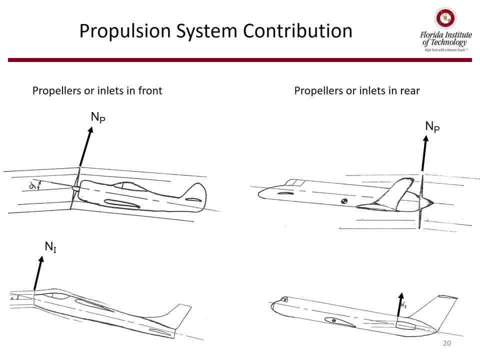 no effect or neutralizing effect or a destabilizing effect. Next, let's look at the different propulsion systems and how they contribute to stability. In the upper left hand corner we see a propeller airplane And generally the way that propeller works, is it? 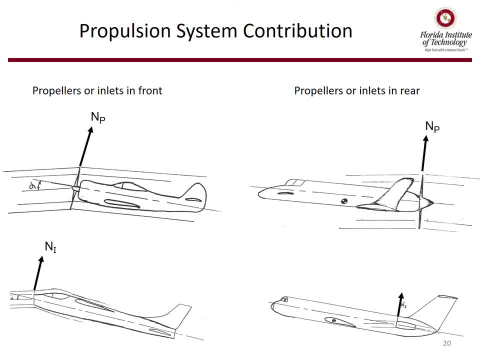 it, it turns the airplane, It's just the air flow and it generates this NP, this normal force. And if you look at where the CG is, say under the pilot's window, or a 25% of the mean aerodynamic cord, 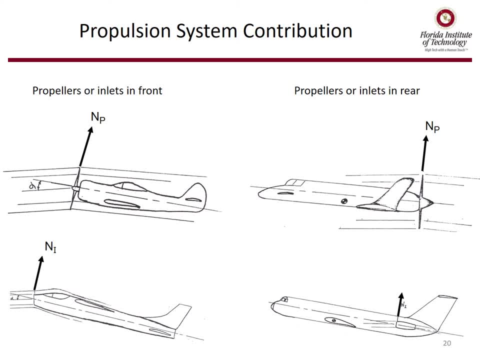 using the right hand rule. that NP then would generate an upward pitching moment. So if you got a disturbance in the angle of attack, it's actually destabilizing. it's going to want to continue the nose to go up. Likewise for the jet in the lower left hand corner. 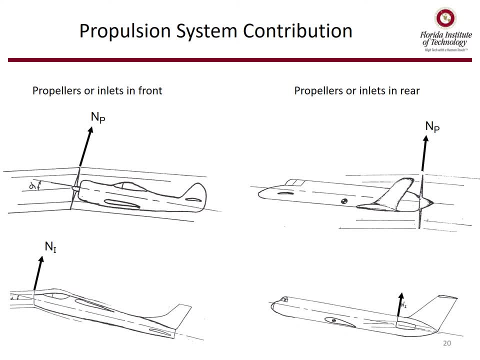 the same thing: the air hits the inlet, it generates that normal force of the inlet which, based on the center of gravity and the right-hand rule, would give us an upward pitching moment or a nose up, and so that would be destabilizing. In the two figures on the right you'll see that when the propeller is in. 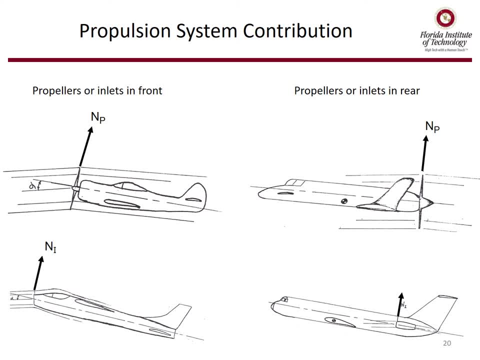 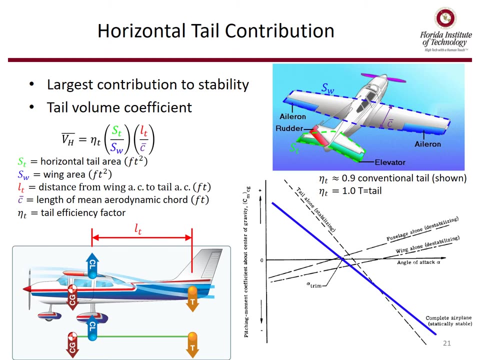 the aft or rear section, or the engines are mounted on the aft or the rear section. it's actually a stabilizing effect, using again the right-hand rule. So we talked about the main wing components, we talked about the propulsion components. 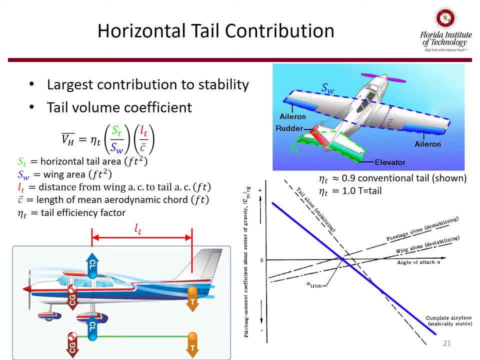 and in the end, it comes down to the tail. The tail is the largest contribution to static stability, or stability in general, and the way you can look at the tail and the effectiveness of the tail is by the way you can look at the tail and the effectiveness of the tail. 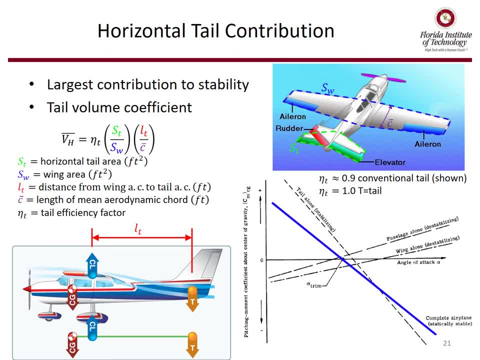 The tail is by a thing called the tail volume coefficient, which we define here as v sub h bar. It's made up of some ratios and a term called a to sub t, and we'll go through these one by one. So s sub t is the horizontal tail area, and it's shown in the diagram here. 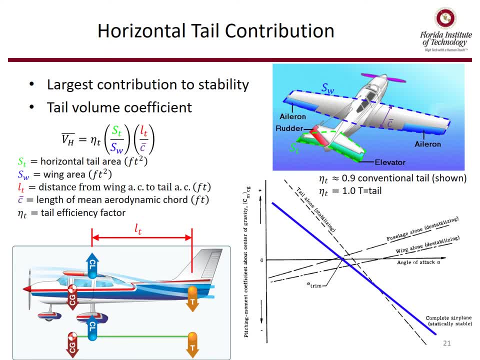 You divide that by the overall wing area. The wing area is always going to be larger than the tail area, so we expect that fraction to be less than one. On the other hand, the next ratio is l sub t, which is the distance from the wing aerodynamic center. 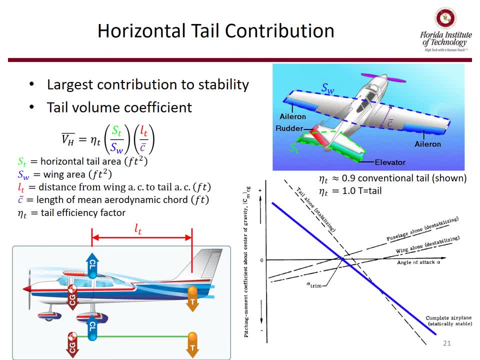 to the tail aerodynamic center. That's a little bit of a large number relative to the mean aerodynamic chord, which is a shorter number. So that ratio is going to be greater than one. And then a to sub t is kind of a tail efficiency factor, and if it's a conventional aircraft like 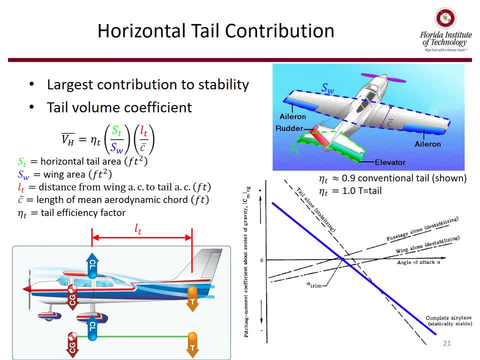 the picture shown, we can assume it to be 0.9.. But if we have a t-tail, where the horizontal tail is in the smooth air, it's not impacted by downwash or other things or propeller effects. So if it's a t-tail, then we can assume that a to sub t is one. 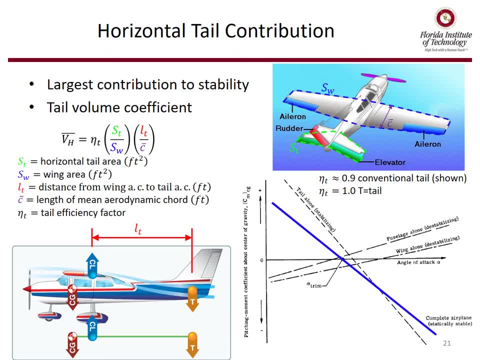 But for a conventional aircraft 0.9 is a pretty good ballpark. So again in the lower right-hand plot we see that that tail is the main stabilizing factor that causes the overall aircraft to be more stable. So that's a little bit of a large number relative to the mean aerodynamic. 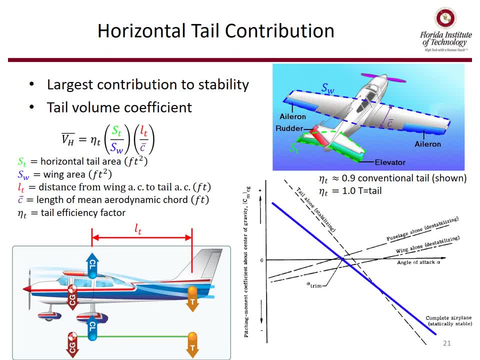 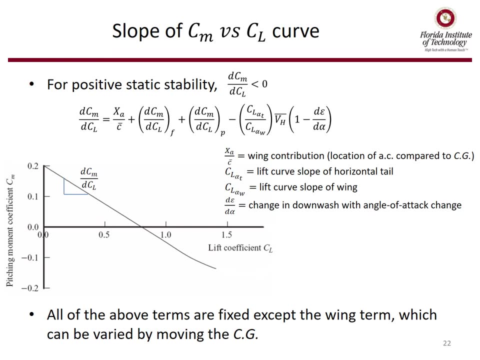 curve. So let's analyze this graph again: CM versus CL, and we have the slope DCM, DCL and it has different components. And so the question is: how do we change the slope or what impacts the change of the slope? 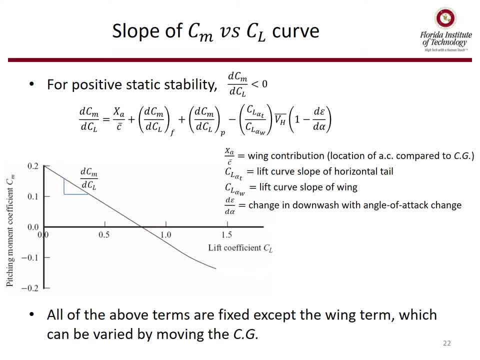 And there's an equation here that shows that we have a wing contribution, which is the location of the aerodynamic center, compared to the CG. We have some propulsion effects. We have the lift curve slope of the horizontal tail ratio to the lift curve slope of the main wing. 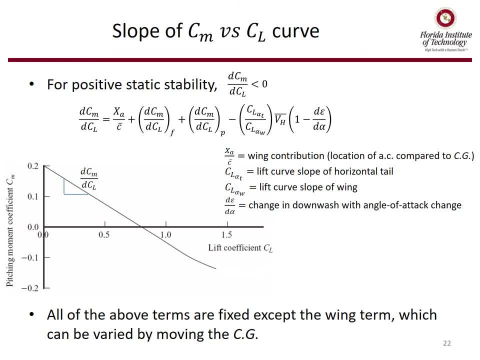 We have that horizontal tail volume coefficient and then we have this d epsilon, d alpha, which is a change in downwash with angle of attack change. So a lot of different things are going into what's impacting the actual value of the slope. But if we really look close, all of the above terms are fixed. 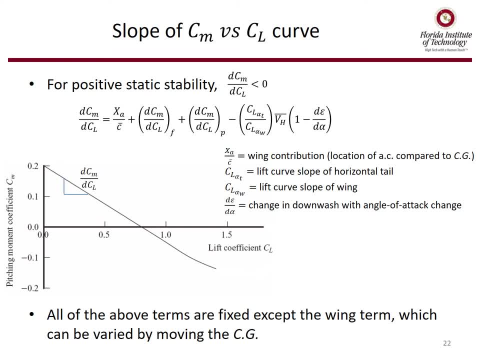 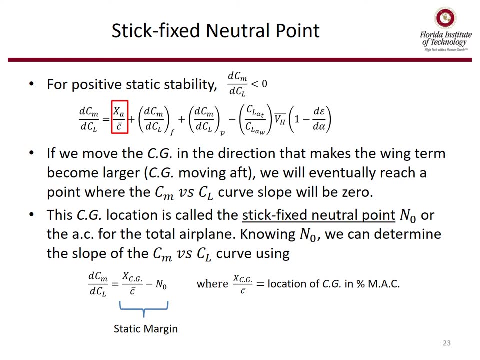 except for that first wing term, that x sub a over c bar, And so we can vary that by moving the CG. Again. for positive static stability we need the overall value of that equation, dcm, dcl, to be negative. 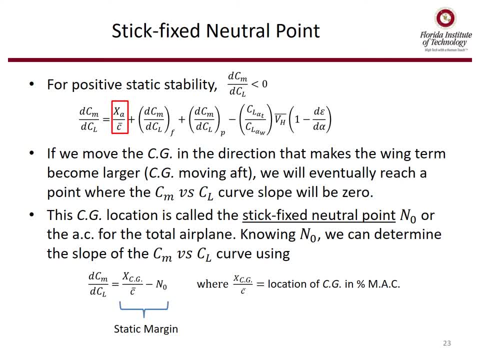 And we're focusing on the wing contribution. So we said we can move the CG in the direction a number of ways. We can move baggage, We can move weights, We can move fuel, et cetera. We can move the CG. 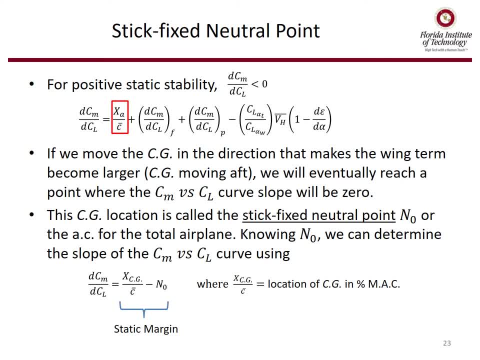 But if we move the CG in a direction that makes the wing contribution become larger, which is effectively moving the CG aft, we will eventually reach a point where dcm dcl will actually be zero, 0. So that slope of that curve will be zero. 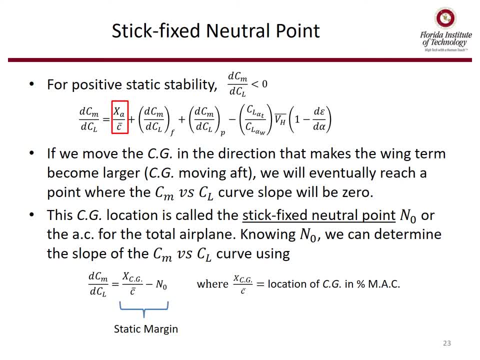 And this CG location, when we move that CG aft back enough to where we get, to that point where the slope is zero, has a special name And we call that the stick-fixed neutral point, given the symbol n sub zero, And what that really represents is the aerodynamic center for the entire airplane. 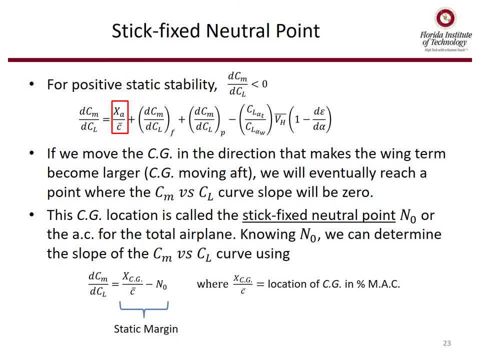 And knowing the stick-fixed neutral point, we can determine the slope of the curve using the equation shown at the bottom. So dcm dcl, that slope is the current CG minus the stick-fixed neutral point And the difference of those two, the current CG and the stick-fixed neutral point. 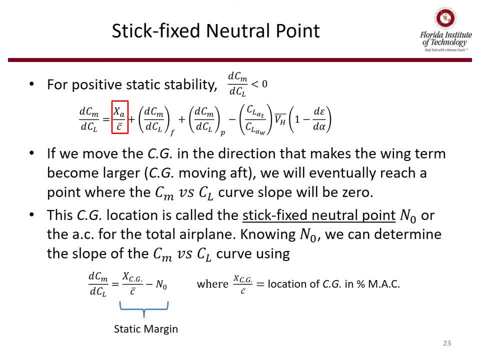 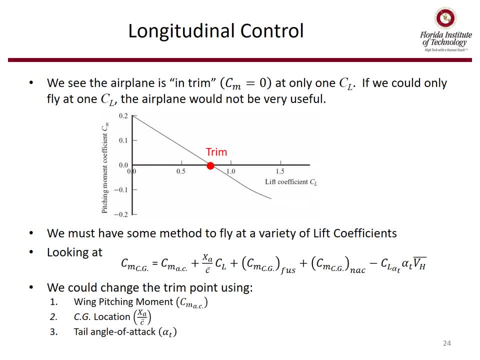 is also given the definition called the static margin. It's the margin of stability. Next we'll switch over to longitudinal control. We've balanced, We've statically stable, but we still need to be able to control the aircraft So we can trim the airplane at zero pitching moment. 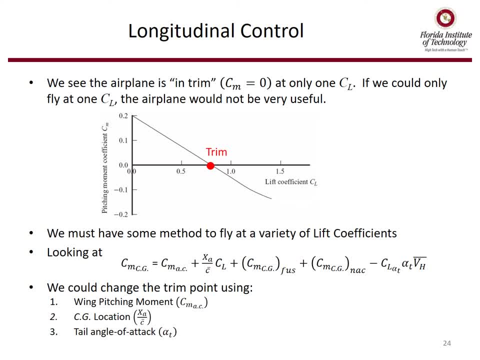 but from the graph we see that only occurs at one cl And that would not be a very useful airplane. Airplanes need to fly at different speeds and different cls, So we have to look at a method of a way to vary the lift coefficient. 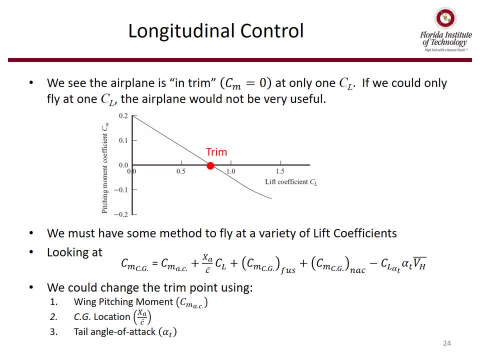 Go back to the equation and we look at the different terms and we say: what can we change? We can move the trim point, We can change the wing pitching moment- the first term- We can change the CG location Or we can change the tail angle of attack. 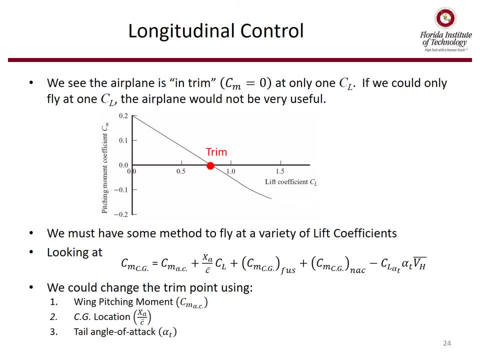 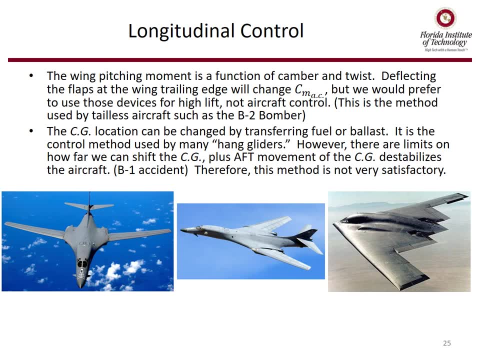 That shows up in the last term. The other things are, for the most part, fixed: The flight direction, the side for flight direction, the direction direction. The wing pitching moment is a function of camber and twist. Yes, we can deflect flaps at the wing trailing edge. 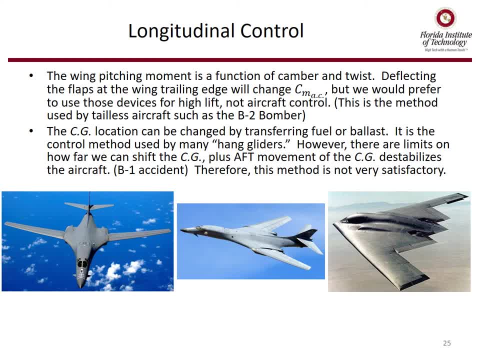 or we can deflect leading edge slats and we can change the coefficient of moment at the aerodynamic center, but we prefer to use those devices for high lift, not aircraft control. On the other hand, if your aircraft is tailless like the B-2,, 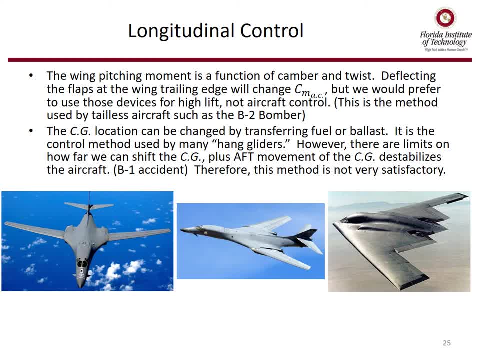 you have to do something with the main wing for control. You don't have a tail. So in that case they do have to use flaps and other devices on the main wing for aircraft control. But for your average aircraft the tail again is going to be the most important part that we use to change our CL. 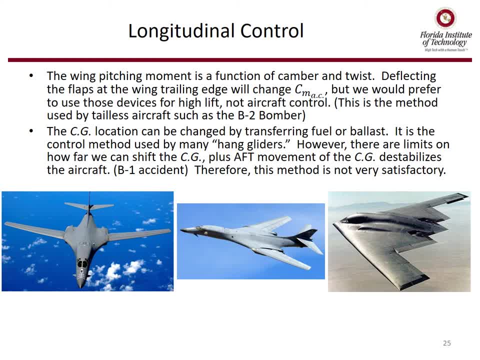 The second method we talked about was moving the CG. We can do that, We can transfer fuel or ballast in flight in real time, but that's not very practical, unless you're a hang glider. If you're a hang glider, you can move your body weight and that moves the CG and gives you a different coefficient of lift. 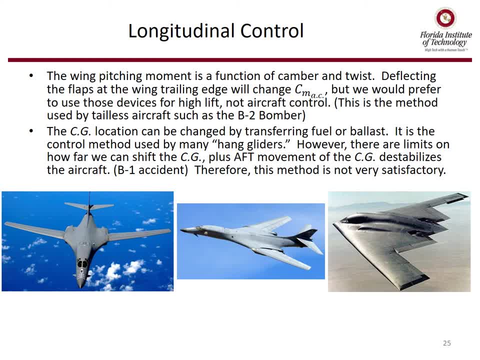 But for real aircraft there's limits And if we move the CG too far, aft we become unstable. In the case of the B-1, that caused an accident early in its development program when the wings were swept from the forward configuration to the rear configuration. 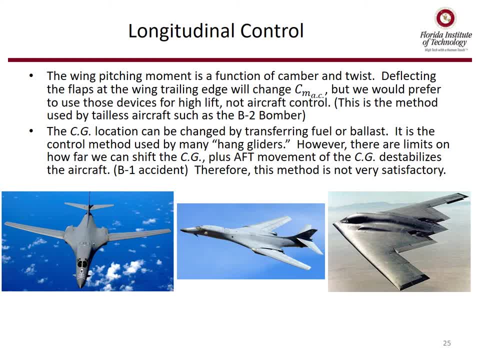 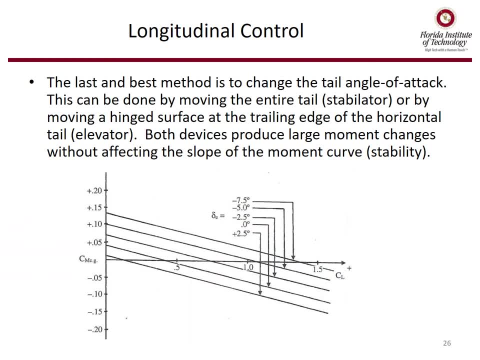 The CG moved too far aft and they weren't able to move the fuel in time to balance it and they had to eject So again. the last and best method to change the CL is to fly at a distance, And we can do this easily by moving the entire tail, which is a stabilator. 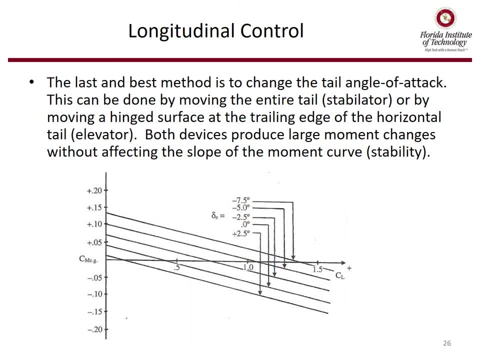 or by moving a hinged surface at the trailing edge of the horizontal tail, which is called an elevator. It all comes down to the horizontal tail. We either move the whole thing or we move the elevator, And both of these devices produce large moment changes without affecting the slope of the CM versus CL or the CM versus alpha curve. 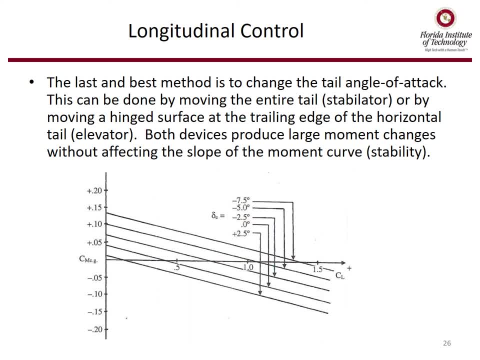 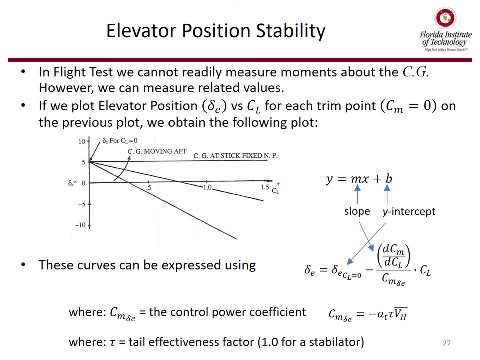 So we get the same stability. but now we get multiple CL positions that we can trim the aircraft and that makes it a usable vehicle. So in a flight test we cannot readily measure moments about the CG. However, we can measure some related values that give us the overall same information. 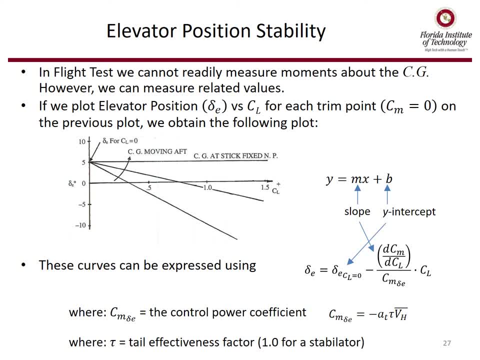 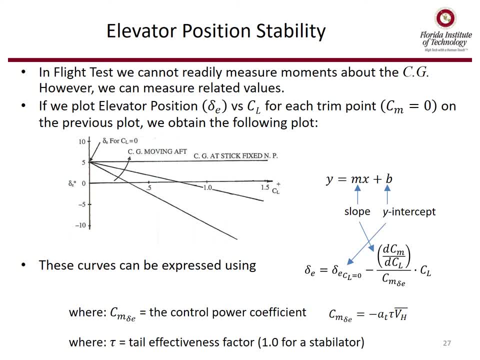 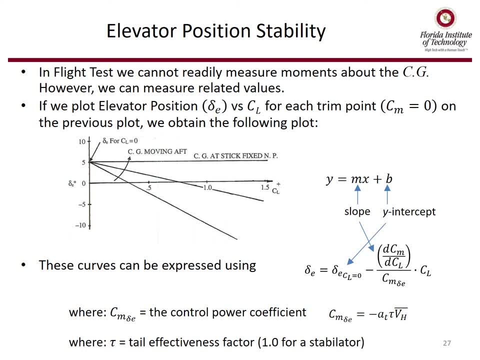 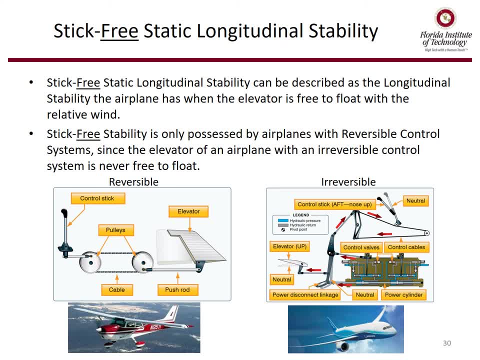 Next, we're going to move into stick-free static longitudinal stability. Next, we're going to move into stick-free static longitudinal stability. Next, we're going to move into stick-free static longitudinal stability. Stick-free stability can be described as the longitudinal stability the airplane has. 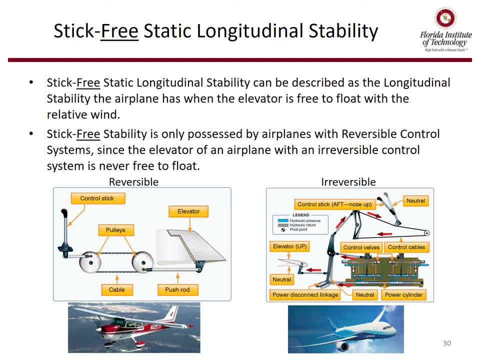 when the elevator is free to float with the relative wind. The only way or the only aircraft that have stick-free stability are the ones with reversible control systems. So, if you remember, back to our introductory lecture in Chapter 19,, we defined what a reversible versus irreversible. 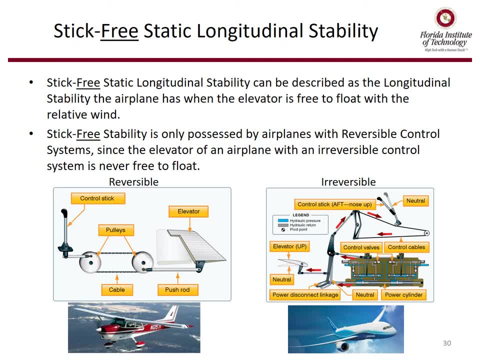 control system is, and I've shown diagrams here to refresh your memory. The bottom line is: reversible means that the stick and the elevator are connected and if I push on the stick, the elevator moves, or if I push on the elevator, the stick moves. 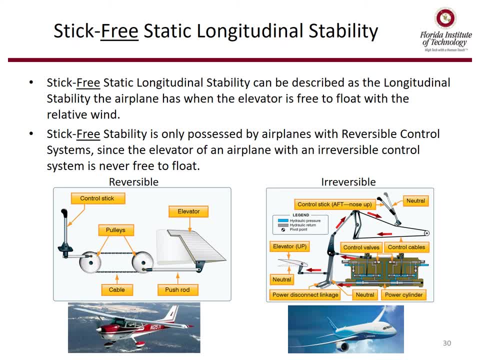 They're connected by cables and pushrods. An irreversible system like the one shown on the right is going to use hydraulics, It's going to use electric motors, fly-by-wire, etc. and so I can move the stick and, yes, that will move the control surface. However, 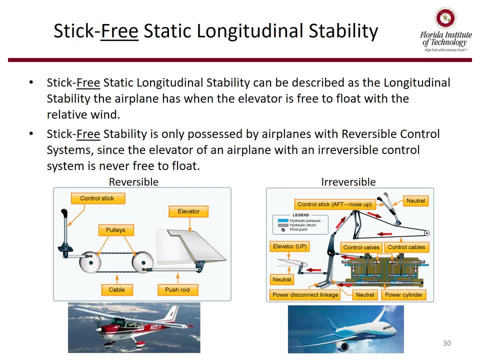 if I move the control surface, the stick does nothing. So that's an irreversible control system. And again, only aircraft with reversible control systems have stick-free stability. because an irreversible control system, the elevator will never float, It's never free to float. 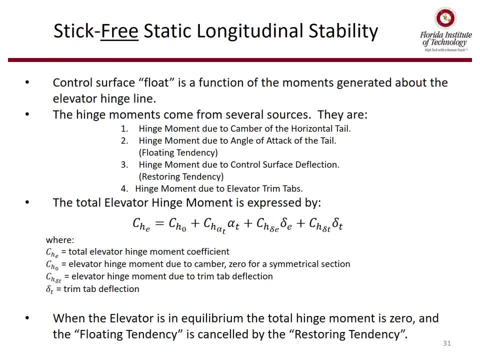 Control surface float is a function of the moments generated by the control surface. If I move the control surface, the stick does nothing. The elevator hinge line. And these hinge moments, they can come from several sources and I've listed a few here. It can be the camber of the horizontal tail, if it has camber. 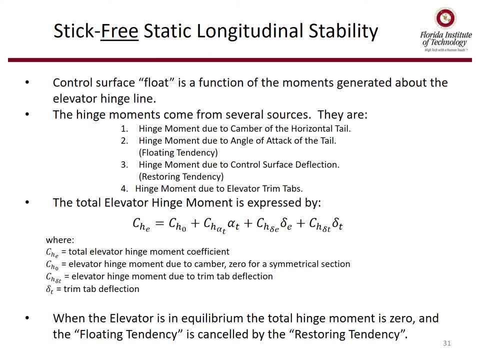 It can be the angle of attack of the tail, It can be the control surface deflection, It can be elevator trim tabs, a number of things, And so we can write one of these coefficient-style equations that sum up all the individual contributions and calculate an overall. 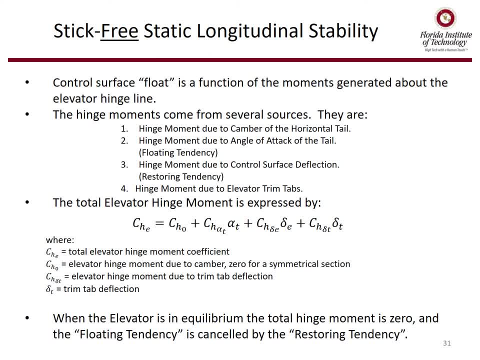 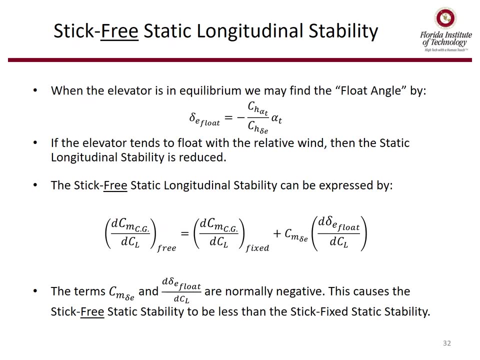 elevator hinge moment, like shown here. So when the elevator is in equilibrium the total hinge moment is zero and the floating tendency happens to be canceled perfectly by the restoring tendency. When the elevator is in equilibrium, we may find the float angle by the equation shown. 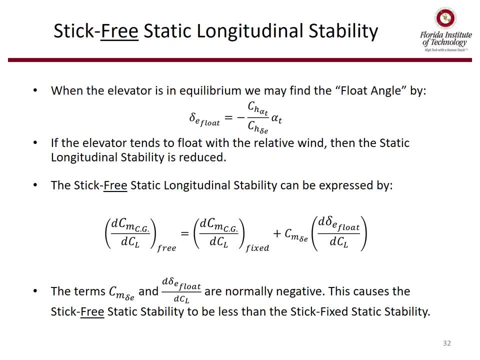 If the elevator tends to float with a relative wind, then the static stability is reduced. The stick float tends to float with a relative wind and the static stability is reduced. The stick-free static longitudinal stability can be expressed by the equation shown here: 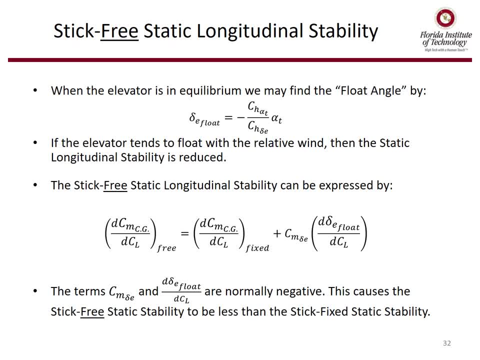 Notice that the stick-free longitudinal static stability has the stick-fixed static longitudinal stability term plus another term: CM. delta E times D, delta E float divided by DCL. Both of the terms on the right-hand side of the equation are normally negative, so this causes the stick-free static stability to be. 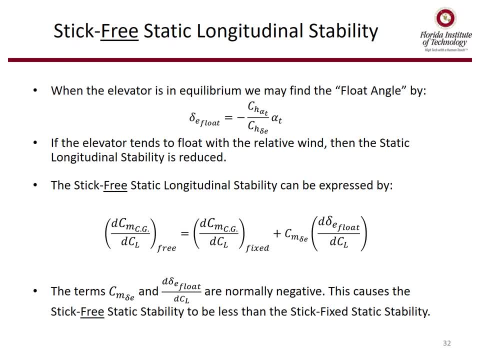 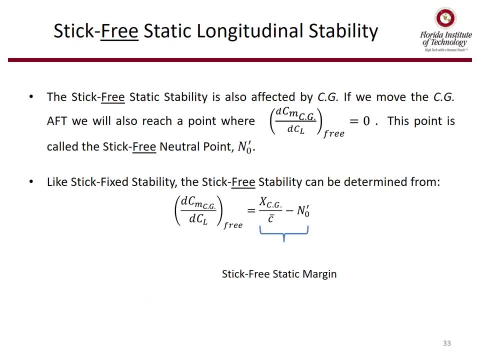 less than the stick-fixed static stability. Stick-free static stability is also affected by the CG location. If we start moving the CG aft, we're going to get to the point where DCM, CG, DCL, stick-free zero, and this point is called the stick-free neutral point, N sub zero prime. 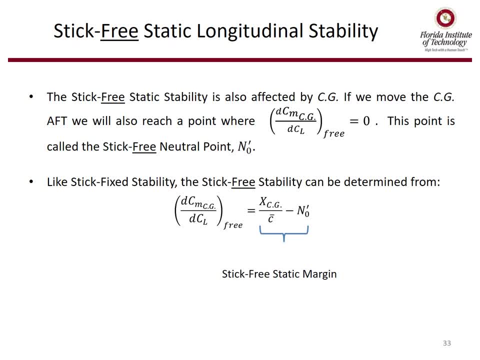 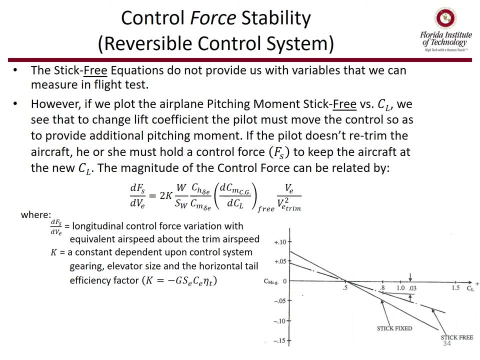 And, just like stick-fixed stability, we can define a static margin that we'll call the stick-free static margin, which is our CG location minus the stick-free neutral point N sub zero prime. These stick-free equations do not provide us with variables that we can measure in flight test. However, if we plot the airplane pitching moment stick-free, we can see that the stick-free neutral point- N sub zero prime- is the stick-free neutral point. We can see that the stick-free neutral point is the check point. We can see that the stick-free neutral point is the check point. 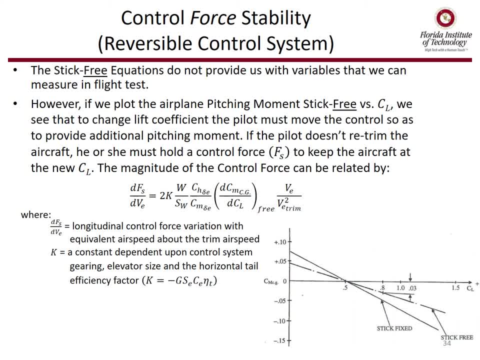 free versus CL. We see that to change the lift coefficient the pilot must move the control to provide additional pitching moment. If the pilot doesn't retrim the aircraft, then he or she is going to have to hold a control force, either push or pull, to keep the aircraft at the 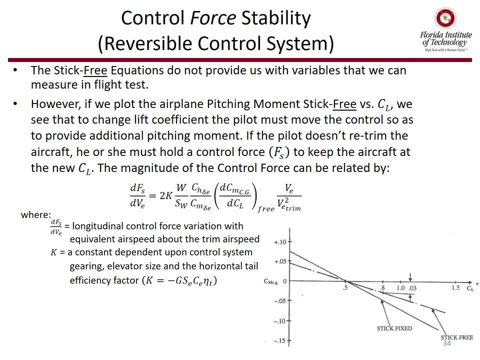 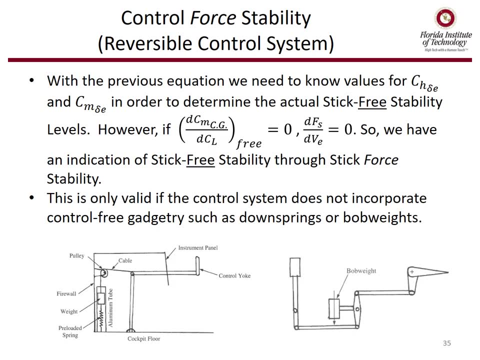 new CL And the magnitude of the control force required can be analyzed with that equation shown With the previous equation. we need to know the values of CH delta E and CM delta E in order to actually determine the actual stick-free stability. However, if we look at the equation 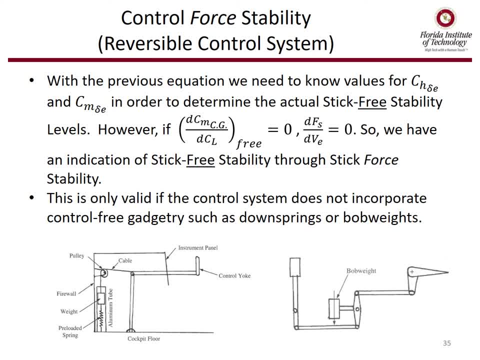 the only way to get DCM, DCG, DCL to be zero is if the change in stick force with equivalent air speed or DFS DV sub E is also zero. So we have an indication of stick-free stability with the equivalent air speed or DFS DV sub E. 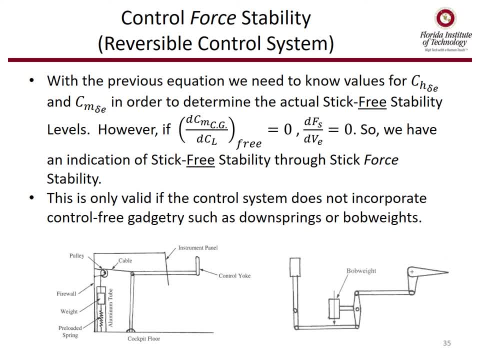 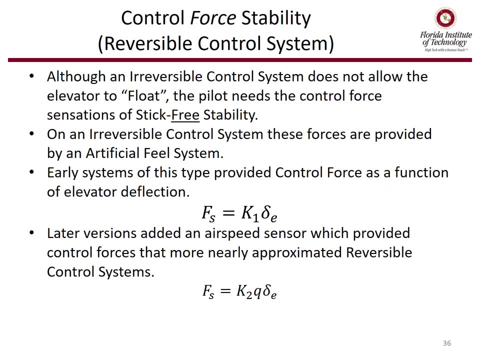 Through stick force stability. However, this is only valid if the control system does not incorporate some of these control-free gadgetry items like downsprings or bob weights. Although an irreversible control system does not allow the elevator to float because the hydraulics or the electronics won't let it, the pilot needs the control force sensation. 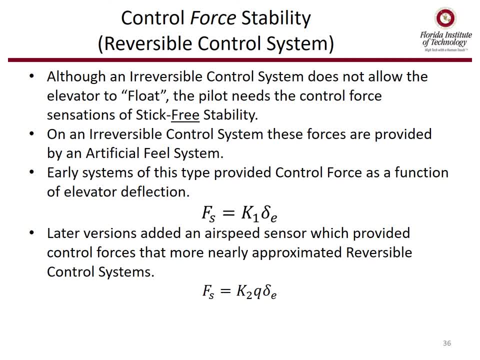 of stick-free stability. So the way this is done on an irreversible control system is through artificial fuel systems. In other words, the flight control system adds force to the pilot so they can feel like it's a reversible control system. In the early times they basically just took a constant K1, some multiple of the elevator deflection. 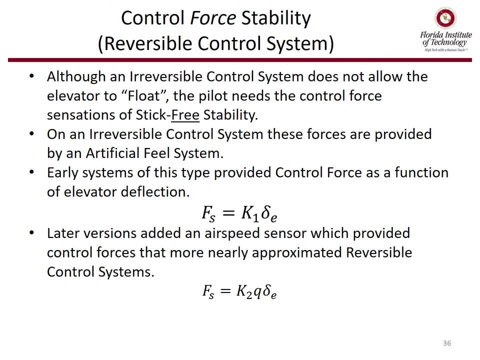 and that was the full control force. So the flight control system adds force to the pilot and that's the force that was fed back to the pilot through the control stick. Later versions they brought in air speed or dynamic pressure so that the different forces happened at different air speeds. 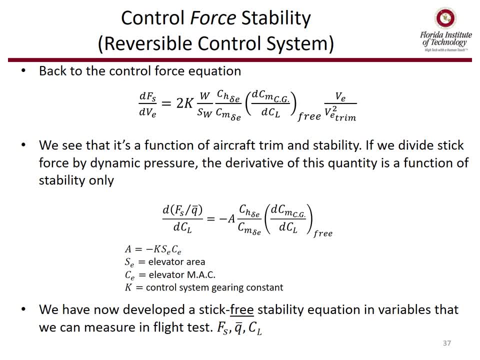 Let's go back to the control force equation: DFS over DVE and then the other stuff. We can see on the right hand side that this equation is a function of not just stability. it also has the aircraft trim information in there, So it's a little tricky to work with. But if we divide stick. 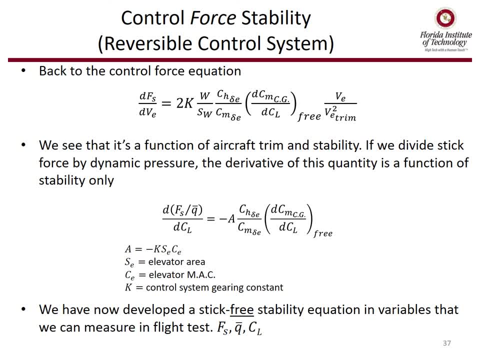 force by dynamic pressure. then take the derivative of this quantity with a function as a function of CL. we get the equation on the middle of the page, And so we see here that most of the parameters are constant, And so the only way to get DMCG, DCL, to be zero is if, on the left hand side, 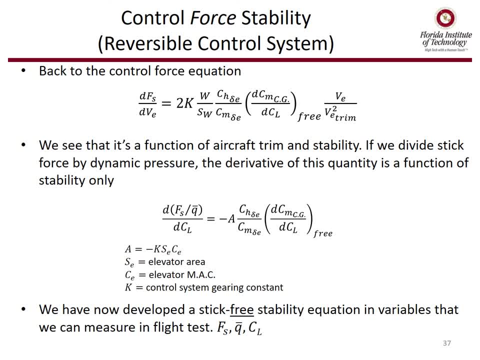 D stick force. So stick force divided by dynamic pressure, divided by DCL, is zero. Now we have something that we can, an equation that we can get, variables that we measure in flight. We can measure stick force, we can measure dynamic pressure and we can measure CL. 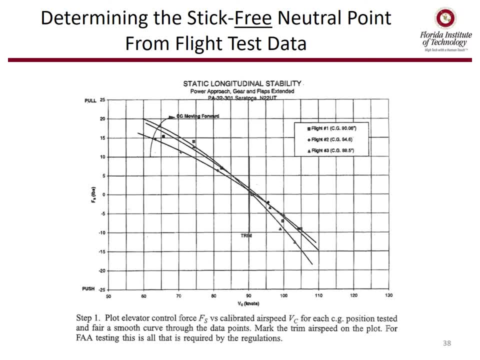 So determining the stick free neutral point from flight test data again, we'll break up the class into three, two or three different data groups and we'll have you guys fly at different CGs: one forward, one mid, one aft. 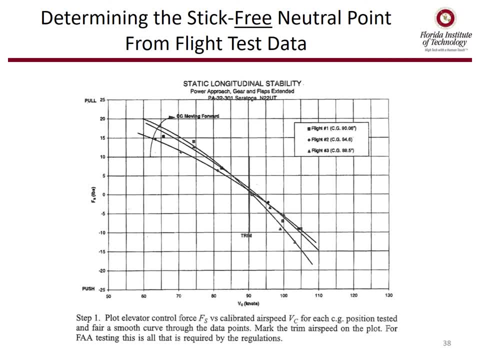 And you'll record stick force data when the aircraft is trim, say in this case, 90 knots. then you'll go lower speeds to 80 knots and to 70 knots without retrimming and you'll have a force. Then you'll go above the trim speed to say 100 and 110 knots, And again the pilot will record. 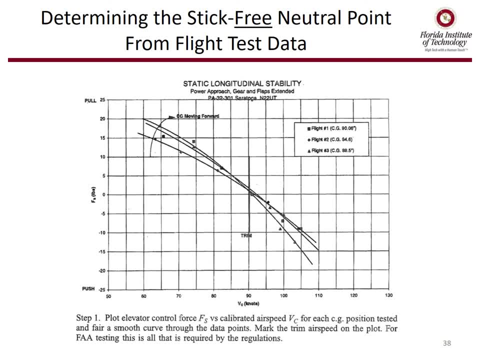 the force. Sometimes it'll be a pull force, Sometimes it'll be a push force, but the raw, the raw data you'll collect in flight after you do the trim is the stick force on either side of the trim: plus or minus 10,. plus or minus 20 knots on either side of the trim. airspeed. 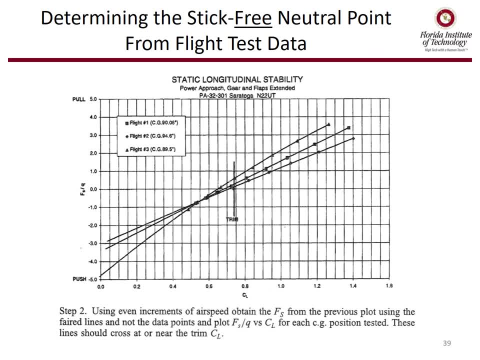 Knowing the stick forces and knowing the speeds, the calibrated airspeeds and the weight, you'll be able to calculate data. now that has our lift coefficient, the lift coefficient on the X axis, and then our stick force divided by dynamic pressure, Q on the Y axis, and generate three of these curves for the difference CGs. 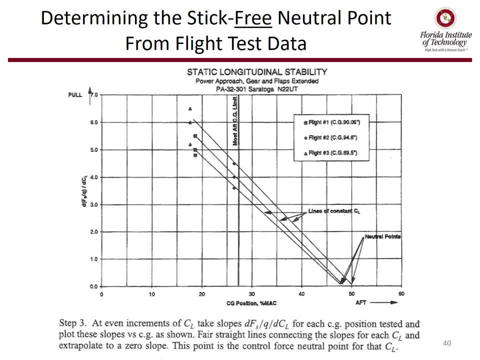 From the previous curve you'll be able to take the slopes or D stick force over Q, DCL and you'll know the CG locations that those were done at. When you have that data you can make this plot. You can then extrapolate that data to where it intersects the X axis, That intersection. 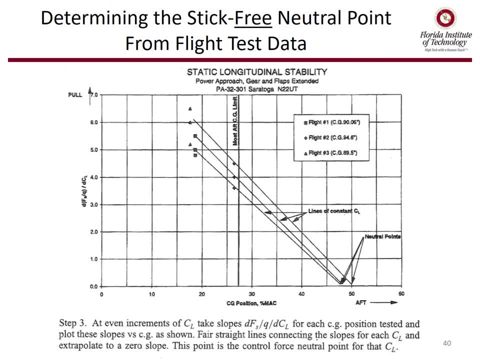 is when D stick force over Q DCL equals zero or the stick free neutral point And you'll get sometimes from the flight data you'll get multiple neutral points and that's okay. You can use the worst case one, but you'll have stick free neutral points when you extrapolate that data to the X axis. 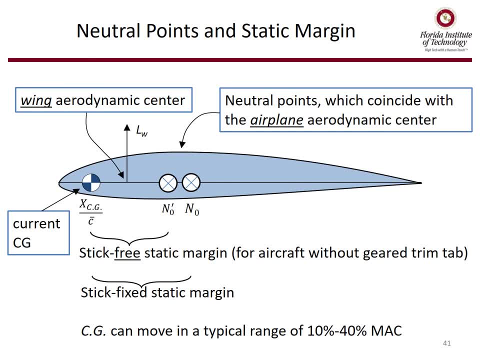 So let's bring all the points of static margin and static stability and stick free, stick fixed, all those things together and let's just look at the wing section. Here's the main wing section. We know that the lift vector acts at the wing aerodynamic center, which is typically twenty-five. 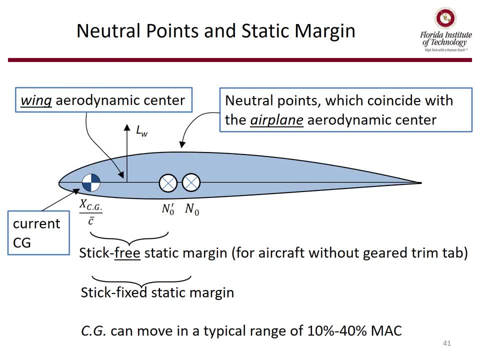 percent of the of the mean aerodynamic chord. The CG right here is shown in a forward location but that can move anywhere from 10 percent to 40 percent of the mean aerodynamic 막. It's just a small variation, This one here, so it's a general tampoco. Theyy can move anywhere from 10 percent to 40 percent of the mean aerodynamic core. 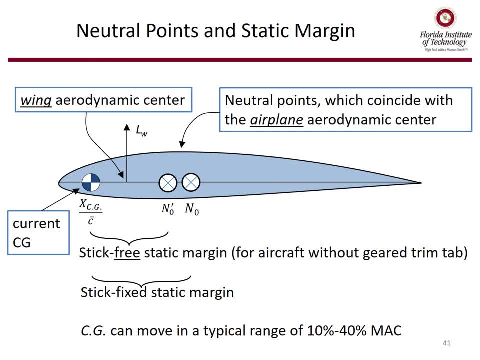 over here in a forward location. no, that can move anywhere from 10 percent to 40 percent of the mean aerodynamic core, aerodynamic cord based on fuel burn, based on passengers, based on luggage, So that's a movable item. The aerodynamic center, though the lift, doesn't move. And so then we calculated different. 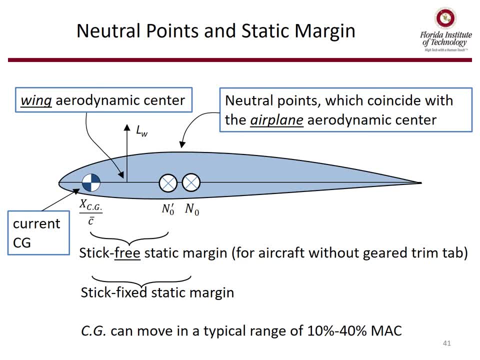 neutral points. We measured those from flight test data and we have either a stick-free neutral point or a stick-fixed neutral point, And then the distance between the CG and either of those two neutral points is called a static margin, And we see here, for an aircraft that doesn't have a gear, 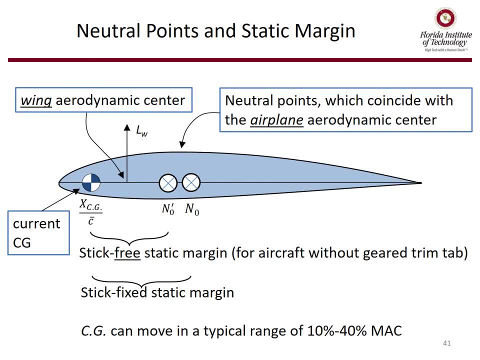 tab or any other gimmick kind of devices, that typically the stick-free static margin will be less than the stick-fixed static margin. And again the neutral points. whether it's stick-free or stick-fixed really is coincident with the airplane. the overall 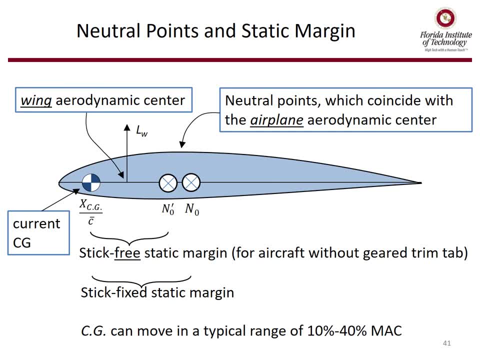 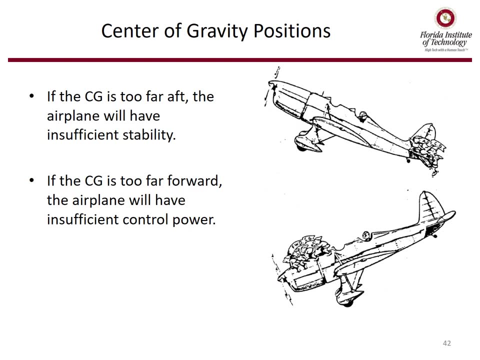 airplane aerodynamic center. Again, the wing has an aerodynamic center, but the wing plus fuselage plus tail is going to produce an overall airplane aerodynamic center and those coincide with the neutral points. So center of gravity positions can be summarized like this: If the CG is too far aft. 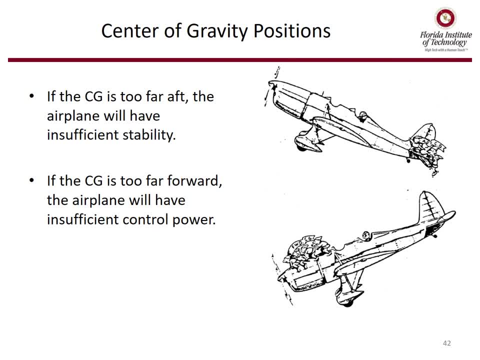 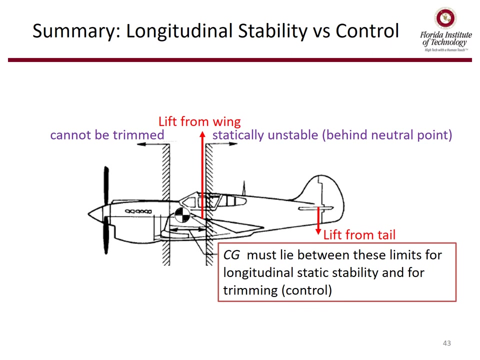 the airplane will have insufficient stability. It'll be unstable. If the CG is too far forward, the airplane will have insufficient control power. So we have to trade off control and stability and we use the CG location as our envelope. In summary, longitudinal stability versus control is shown here Again, the forward. 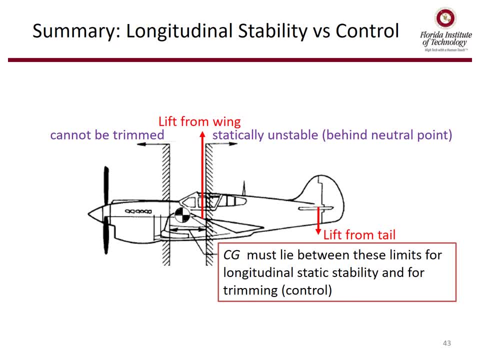 CG limit means I cannot trim the aircraft. The aft CG limit means I'm statically unstable, So our CG then needs to reside in between these two boundaries for the airplane to be both statically stable and trimmable.